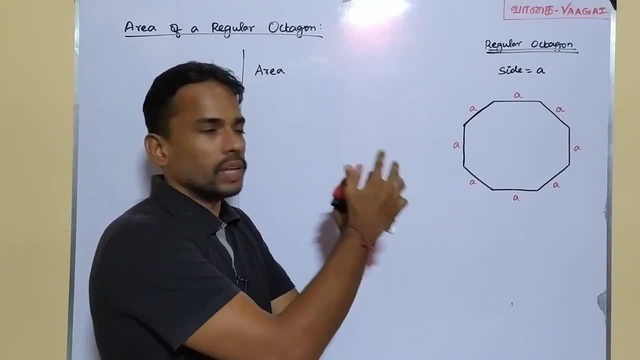 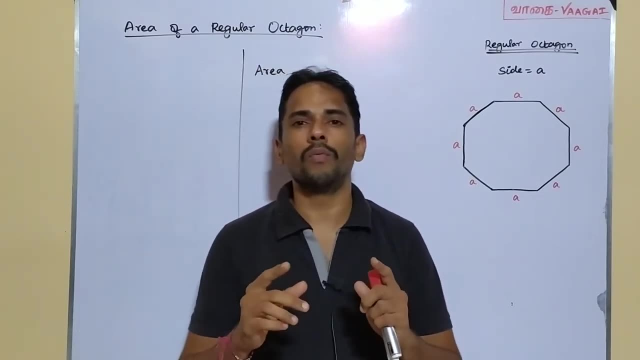 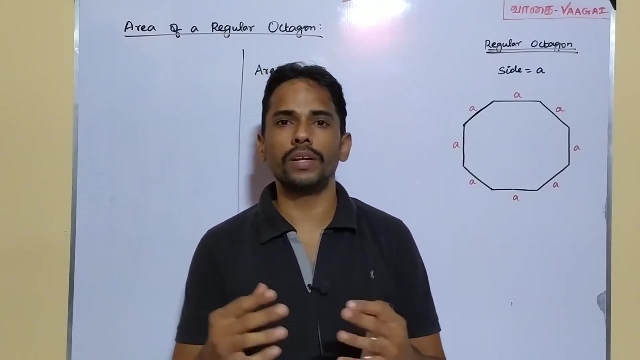 to find the area to solve and get the formula to find the area of this regular octagon, The approach that would be definitely helpful for you. That's an assurity given here. So for that reason I kindly request you to watch this session, this video, till the end, so that you would get a good information. 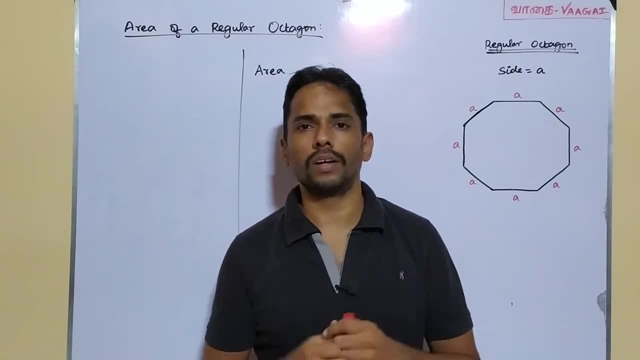 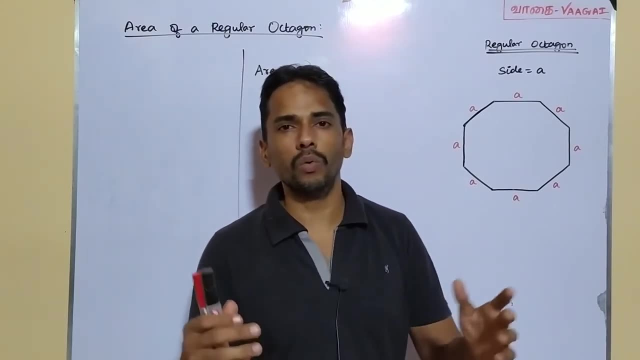 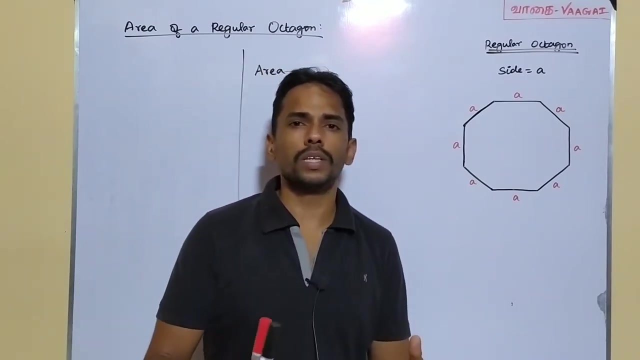 That's fine. Yes, we start with our thing. So, yes, here we have a regular octagon, and whose area is what we are going to find, And, before that, what is a regular octagon? What is an octagon? first of all, An octagon is a polygon. 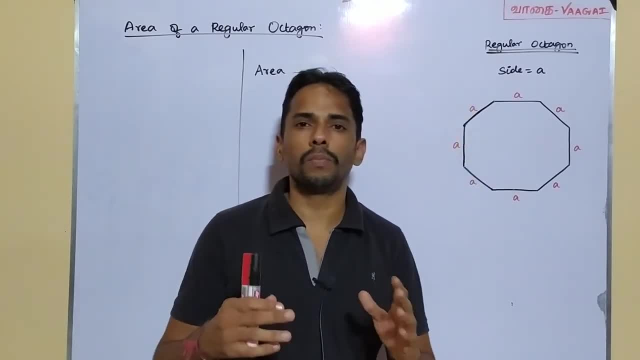 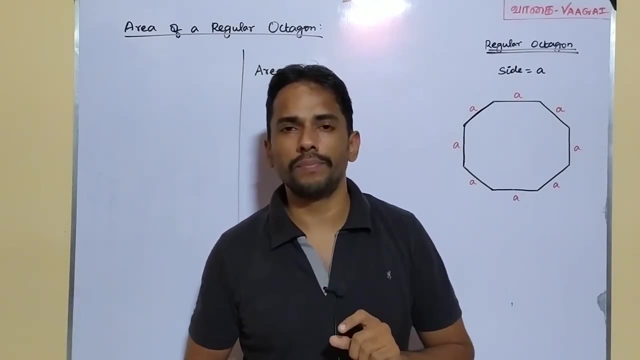 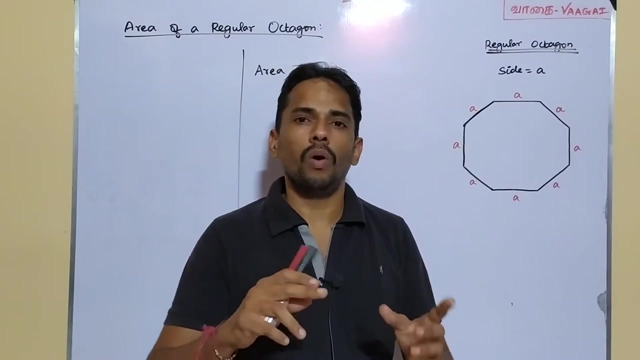 which is having eight sides. Such a polygon is what we call it as a octagon. And here, what makes it to be a regular octagon, if you ask? It's very simple: For an octagon, for all its eight sides, we have eight sides, So when all its eight sides are equal in length and also at the same time. 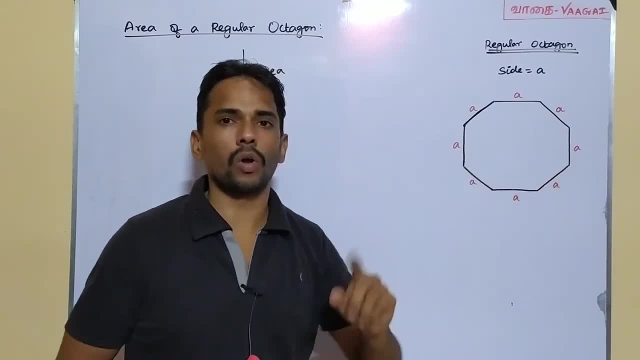 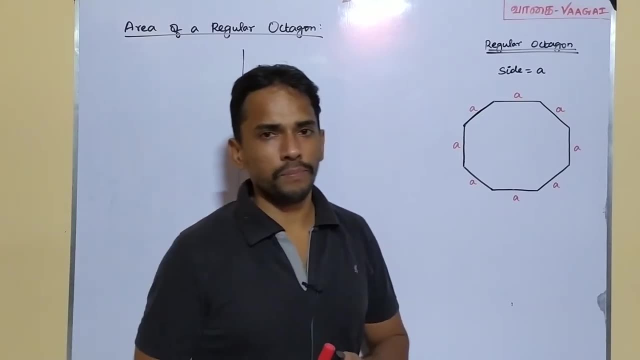 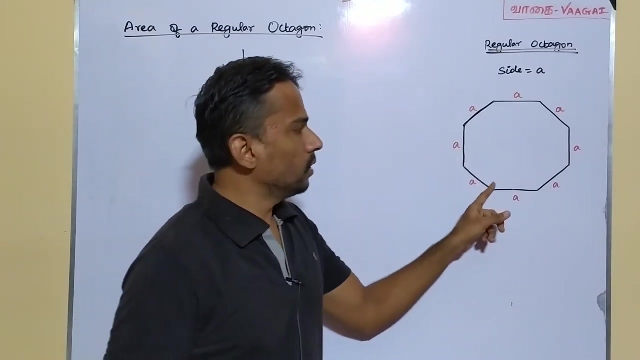 all of these eight interior angles that we see here are also equal. then we end up with a regular octagon. So here is a regular octagon, and here we have taken the side, each side, of this regular octagon, to be A, And here these interior angles are also definitely equal, For this octagon is: 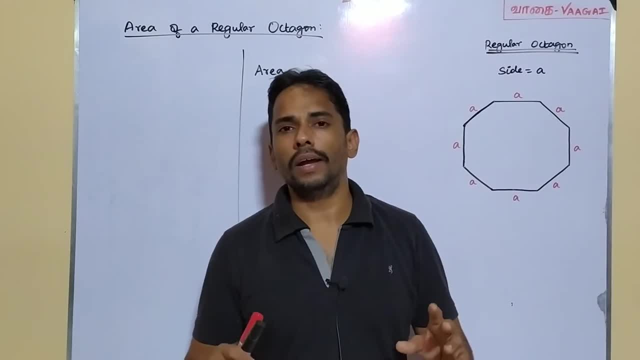 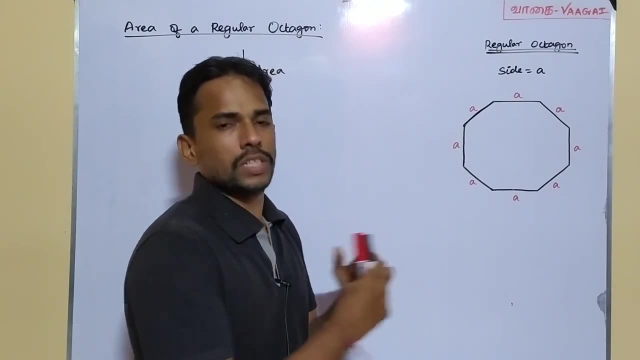 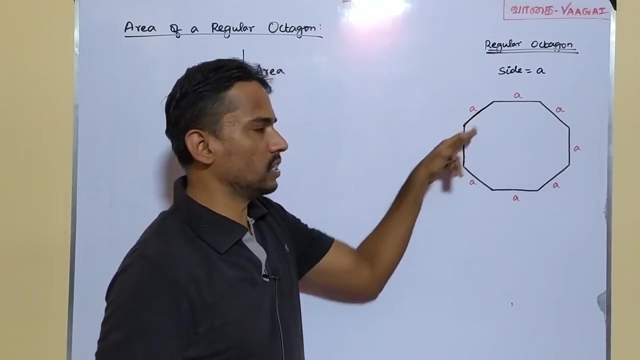 what we are going to find the area. And next thing is we are going to take some approach to find the area. But before that, as we just discussed I just told you: now, right, All of these interior angles, I mean each of these angles we see here, they are going to be equal. Let's try to find this interior. 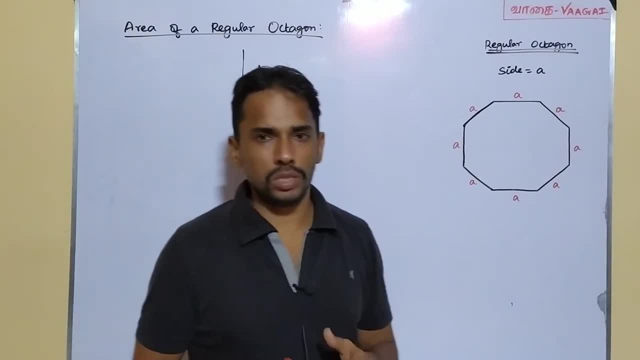 angles first. then we go find the area. Why? Because on the way of finding this area, we may have to use this angles property. that's the reason Let's try to find the angle here itself. then we go find the area. Yes, fine, okay. 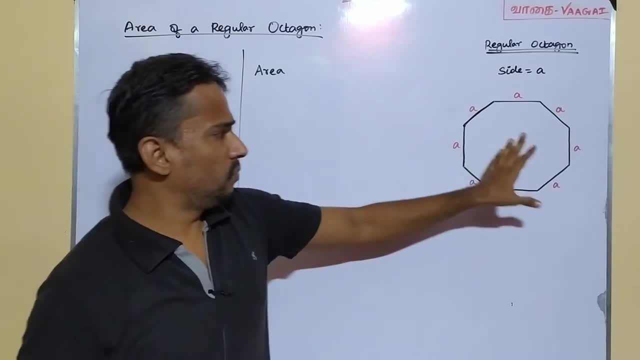 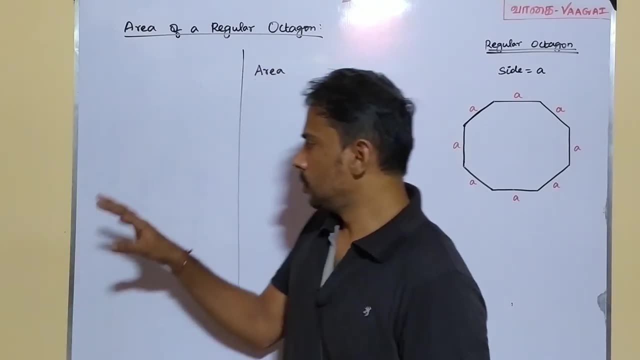 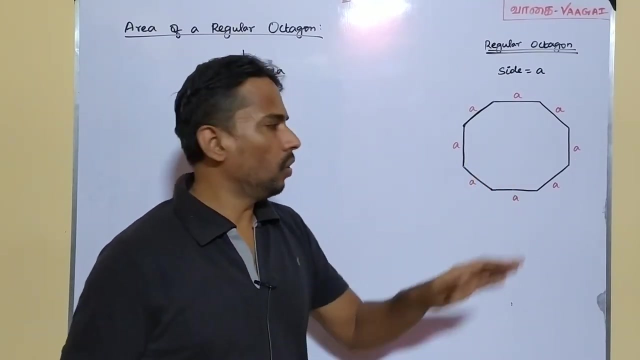 Yeah, And one more thing. Let's take the figures elements here, Let's take the working area here, And if any rough calculations or anything is needed, let's use this space to work them. Fine, yes, So now let's try to find the interior angle of this regular octagon. Let's do with this, So for. 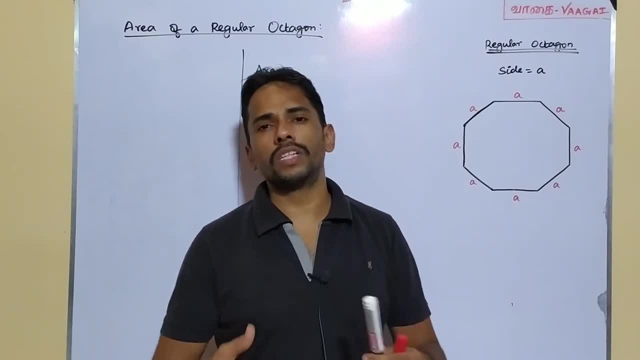 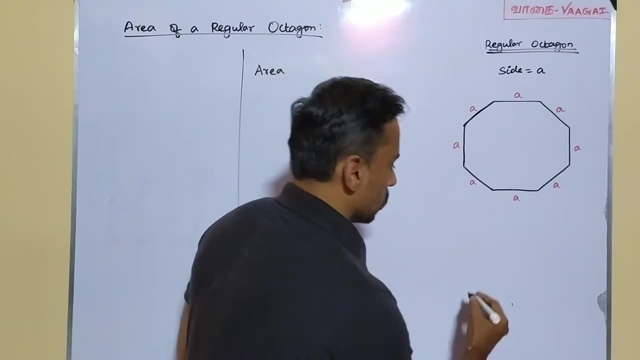 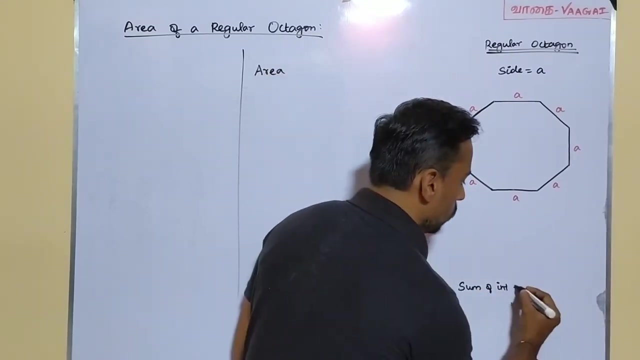 any polygon, the sum of interior angles will be equal to. it will be equal to. we have a formula right, So let me use this font space here. So sum of interior angles of any regular octagon will be equal to. for any regular polygon will be equal to 180 times of n minus 2.. So 180 degrees. So here: 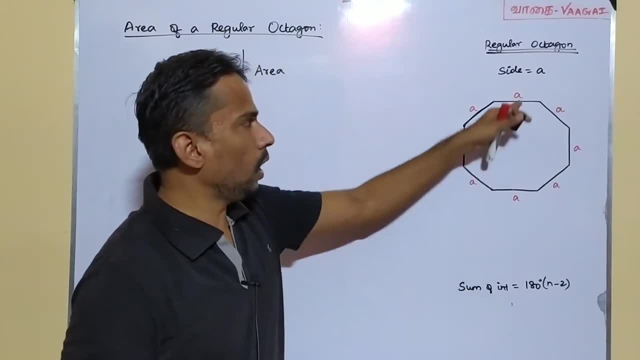 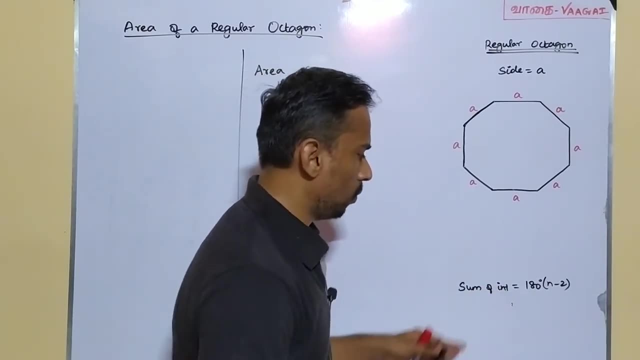 this n stands for the number of sides. And now our polygon is nothing but an octagon. So for an octagon, the n value is 8.. Is it or not? So for octagon, the sum of the interior angles will be equal to 180 times. 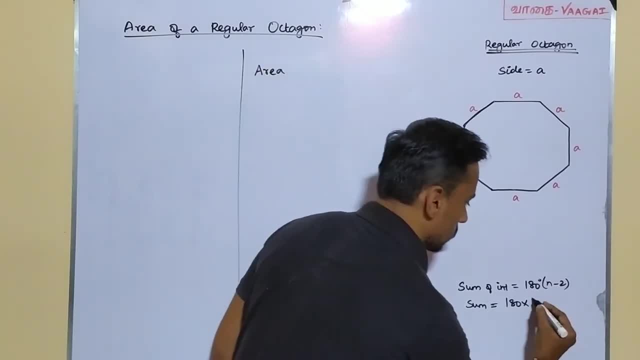 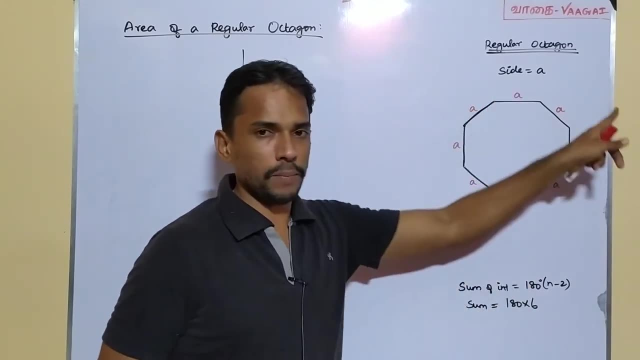 What is n here? n is 8.. So 8 minus 2 will be 6 here. Yes, put it. But this 180 times 6 stands for sum of all these angles. I mean sum of all these 8 angles we see here. But if we need each of these, 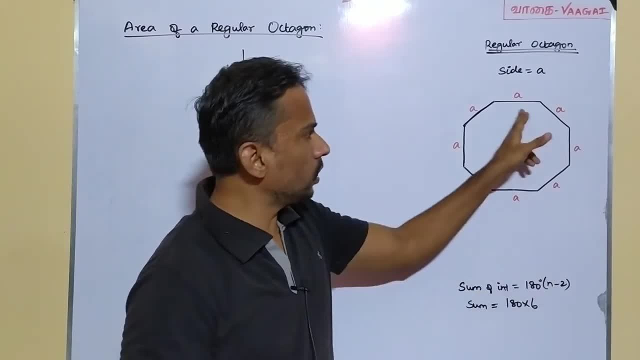 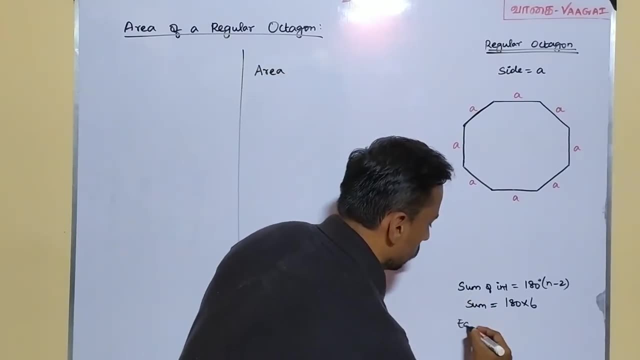 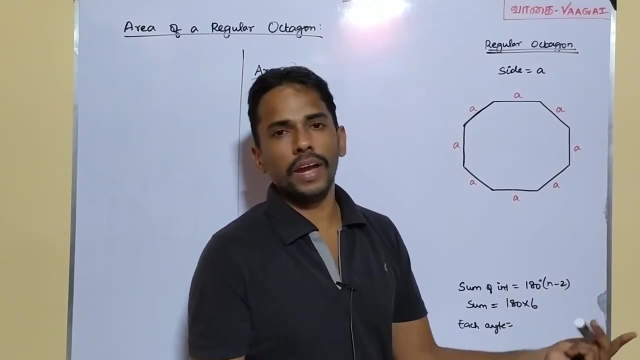 angles. what has to be done? Just now we saw, we know that all these angles are equal And in that case, if we know, if we want to find each of these angles, So each angle will be equal to, it will be equal to this product 180 times 6 divided by 8.. That's it, Because we know that there are 8 angles and all of 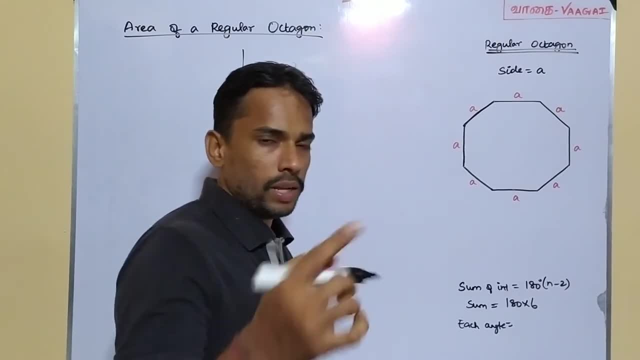 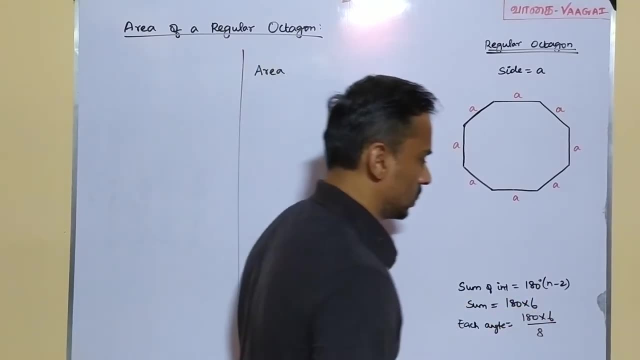 them are equal, And 180 times 6 is the sum. And if we want each of these angles, just divide this 180 into 6.. This product by 8. So 180 times 6 by 8.. So we can just simplify this: 6 and 8. We can make. 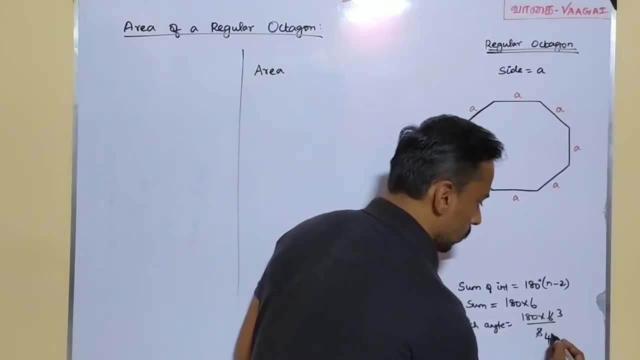 it as 3 by 4.. So we have 4 and 180.. This will be 45 times, And 45 times 3 will be equal to 135.. Is it or not? So this will be 135 degrees, And that means each of these angles we see here. That means this: 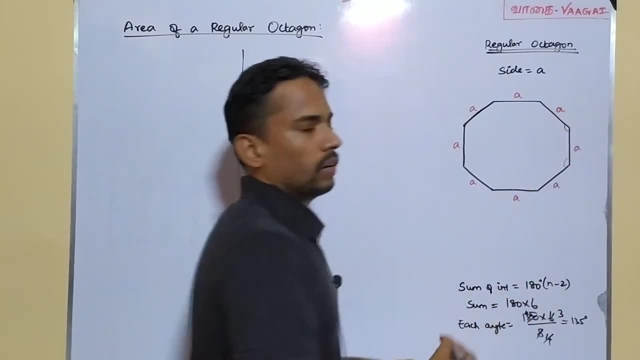 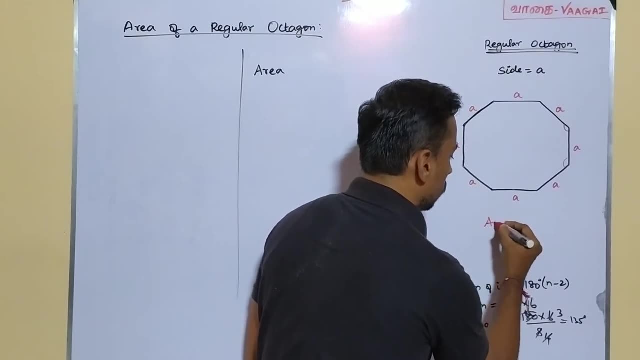 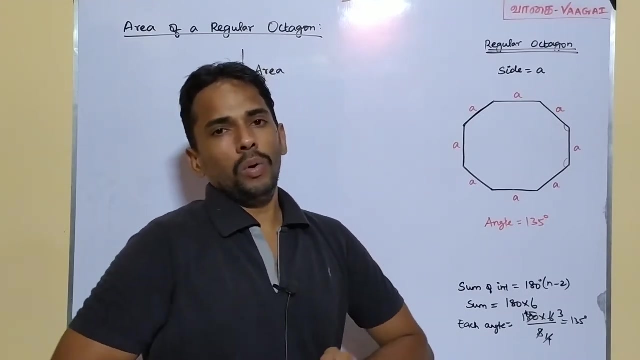 angle, This angle, This angle, Whatever All these 8 angles, Each of them are going to be exactly 135 degrees. Let's make a note of that. angle is equal to 135 degrees. Yes, our first part is successfully over. Now it's the time for us to get into the areas, part For which let's try to make. 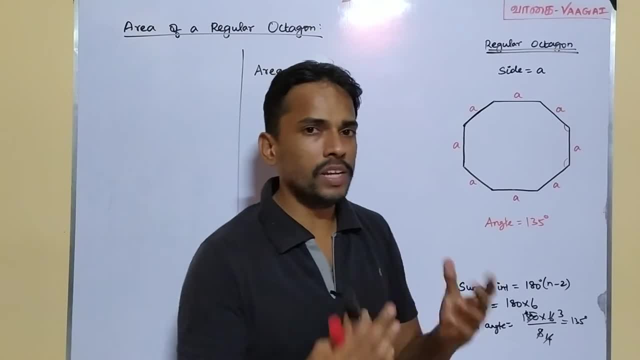 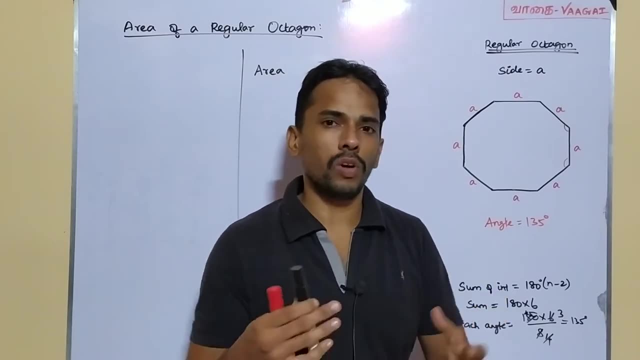 some kind of adjustment- Adjustment here, Or some kind of partition here. We will try to partition this octagon in a particular way, such that it will be very easy for us to follow and then get the area. Fine, Yes, Ya, we go, So I'm. 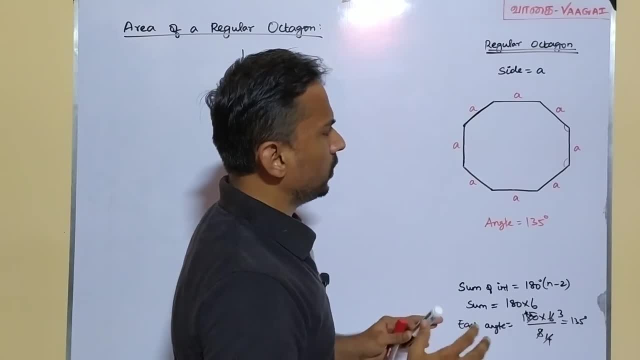 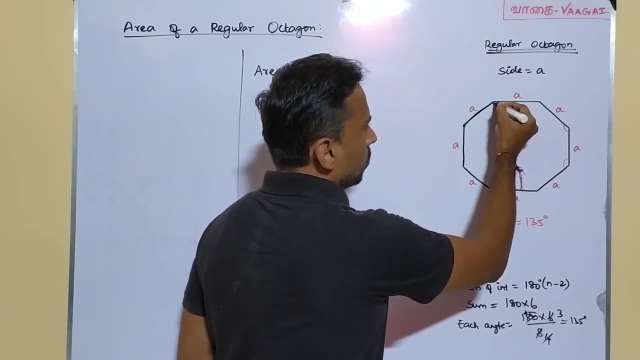 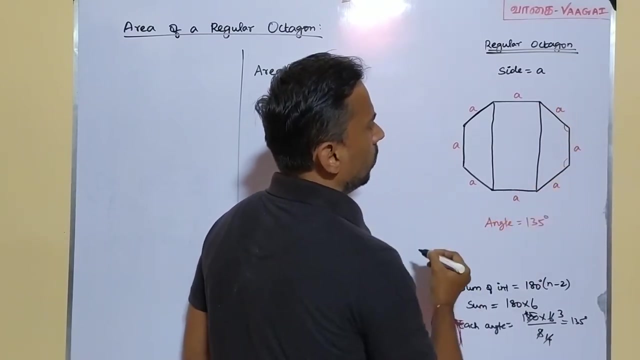 going to just going to split this octagon in a particular way. Let's have a close look how we are going to do that. So just draw lines like this, Like this, A line like this, line like this, and then, trying to connect these two vertices, a line like this and another line. 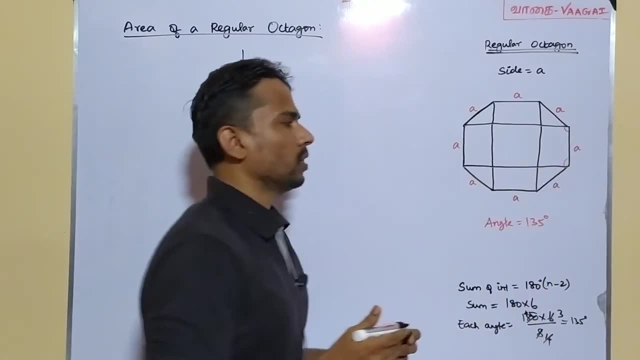 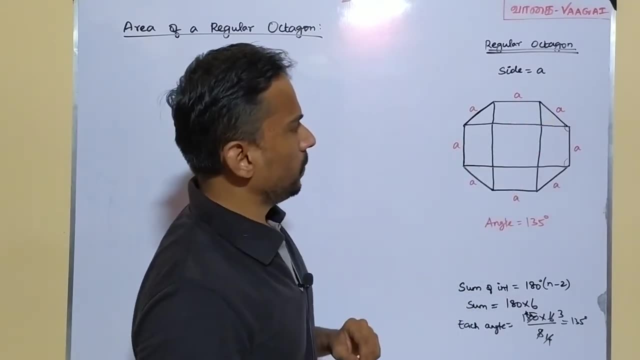 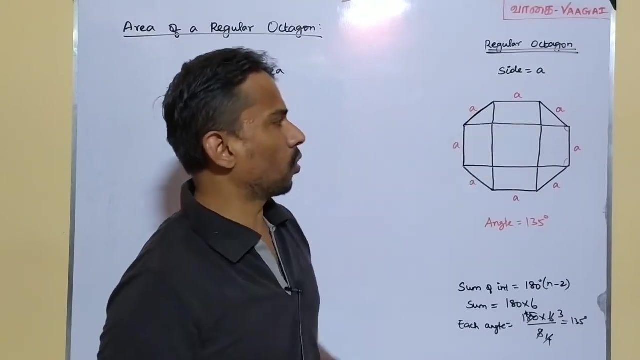 like this: yeah, this is really enough for us. so now, if you have a close look, we have divided our octagon like this. so that means, can you just count and see how many regions are here, or how many regions that we can see here inside this octagon? so if you see that there are one, two, three, four, 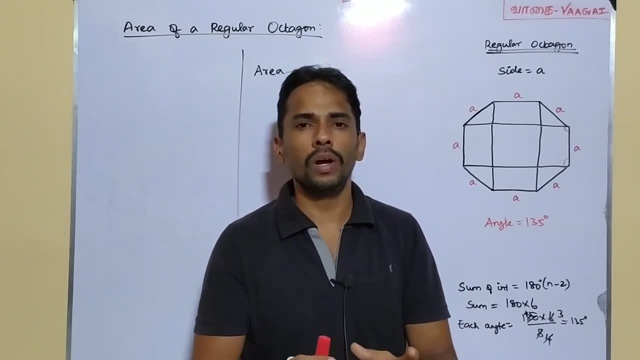 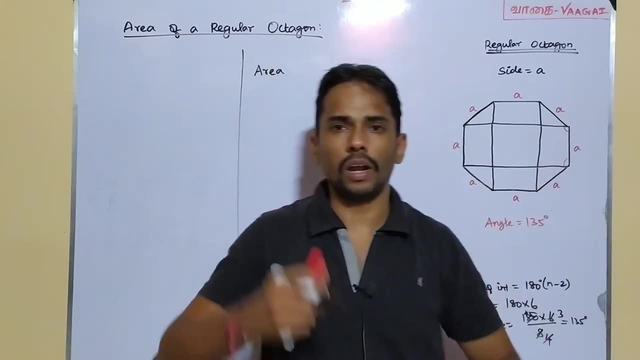 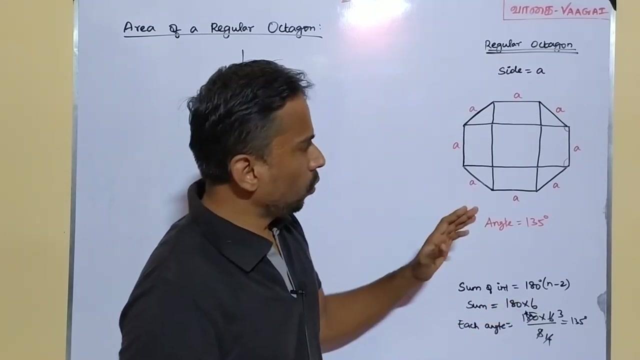 five, six, seven, eight, nine. our octagon got split into nine regions inside, so that means these nine regions sum is what are octagon's total area finished, right, yeah, next is now again. we'll have a close look. we'll try to identify what are all the shapes we have inside this octagon. right, yes? 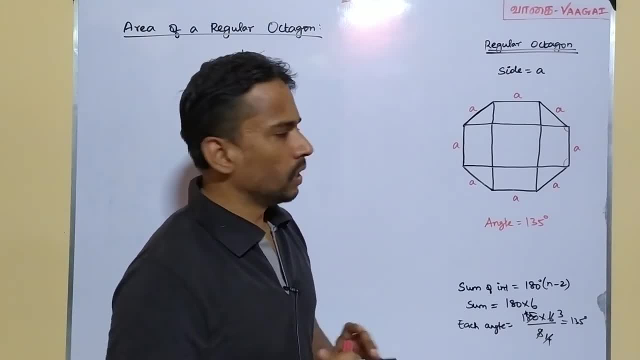 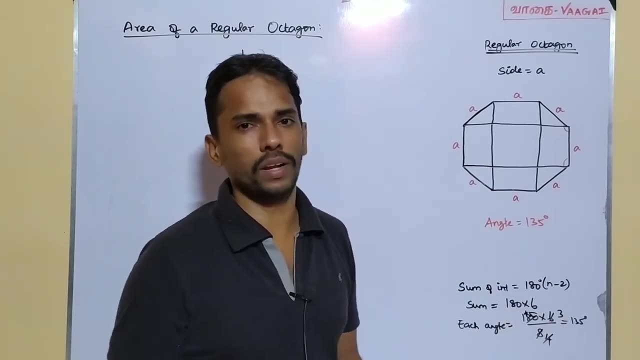 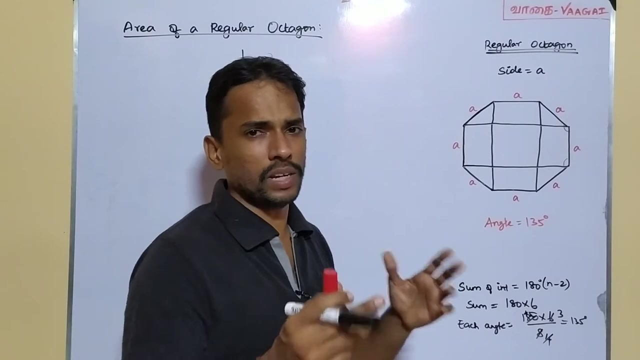 fine, yeah, so it's very obvious that the shape that we see here at the middle, the innermost one, is octagon, obviously going to be a square, no doubt in that right. so we have a clear square here. yes, and you may ask how it is a square. it's very simple for us to understand and observe here. see here, just try. 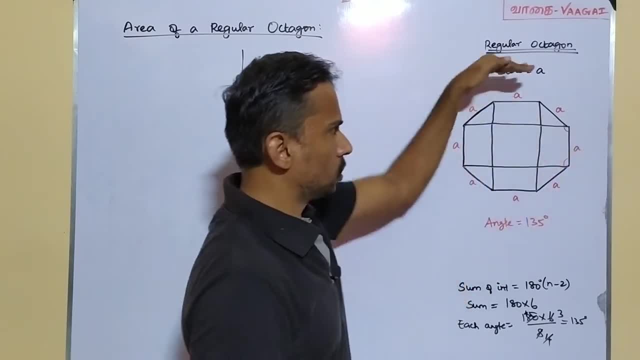 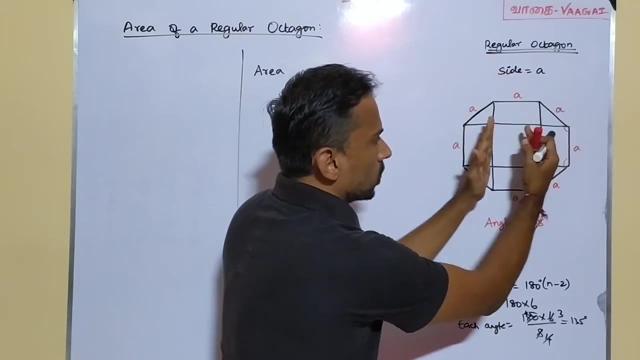 to project these sides here, these four sides here i mean this top, this left, this right and this bottom. just see all those four sides, just get them projected inside. so what happens is you'll end up with this innermost shape, which will be none other than a square, is it or not? 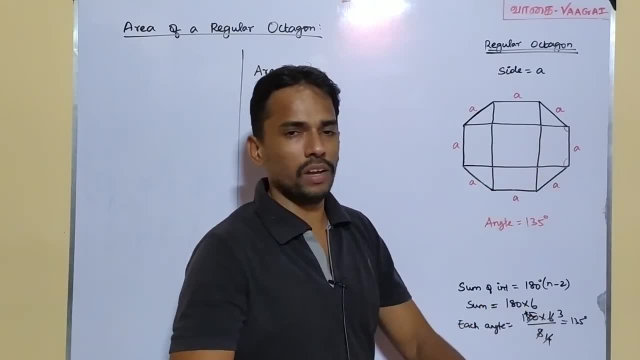 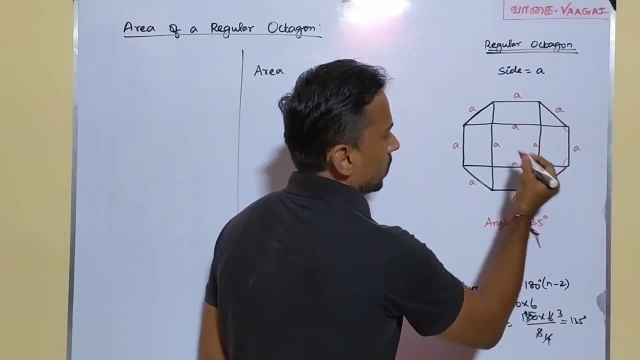 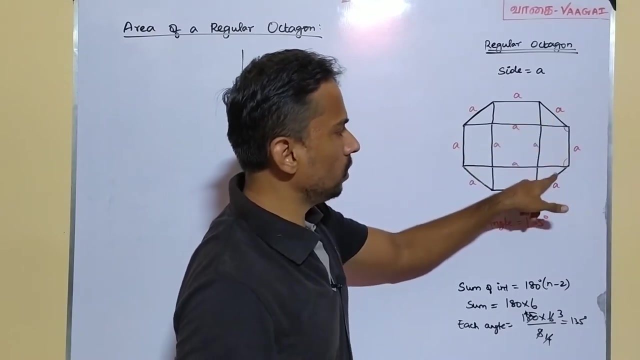 so that means we have a square. and again one more thing: we can say very easily that the square will have side equal to a, is it or not? yes, so we have one square that we can see inside. and now next is: let's see the corner portions. here we have four triangles. and another thing is: let's have a look. 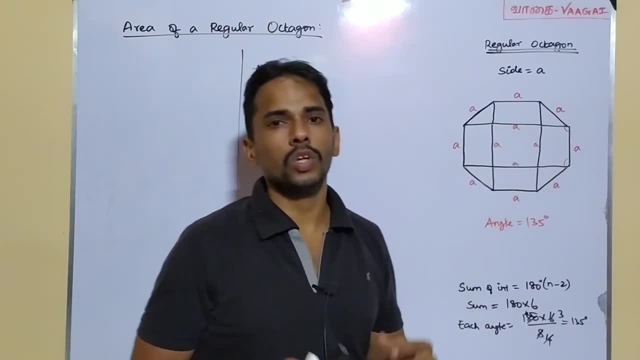 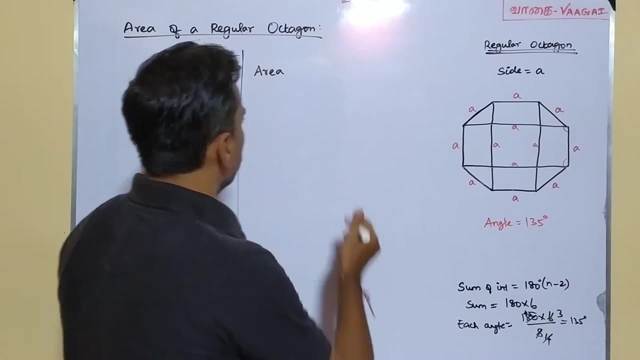 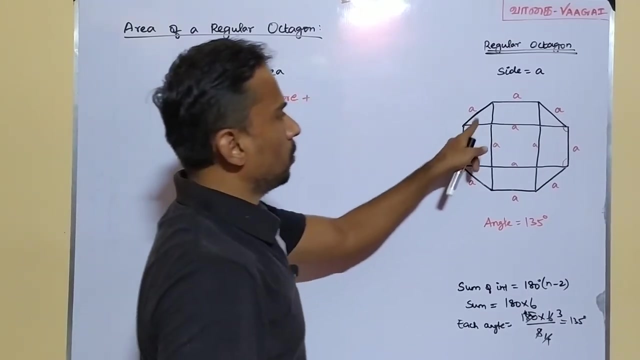 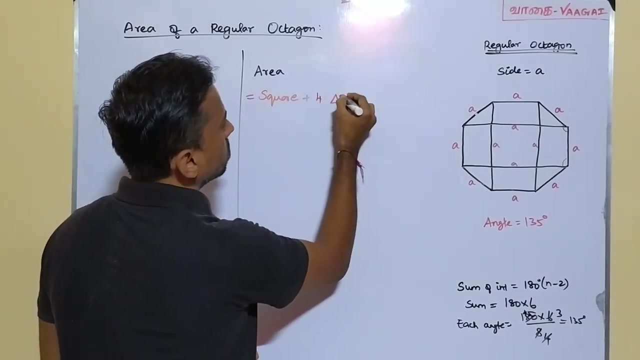 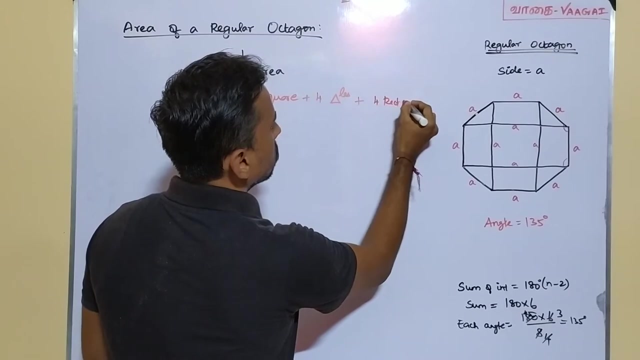 on these shapes. we have four rectangles, so that means it's very, very clear that area of this octagon is none other than sum of this innermost square, so square plus sum of this four triangles, this four triangles area also that has to be added right. so four triangles, that one plus, and we have four rectangles here, so four rectangles. so when we 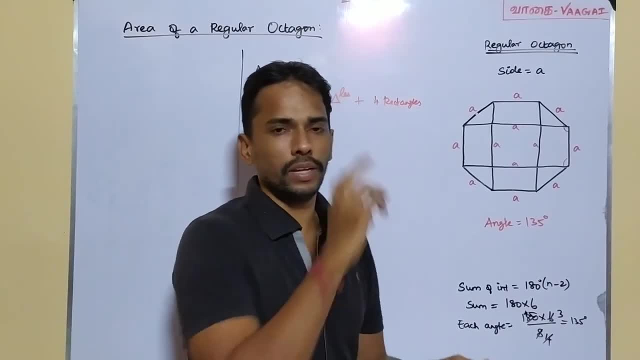 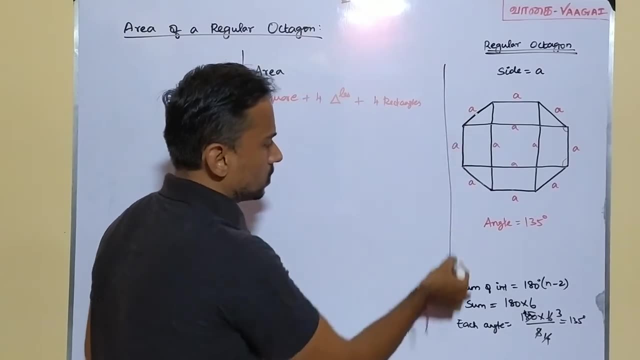 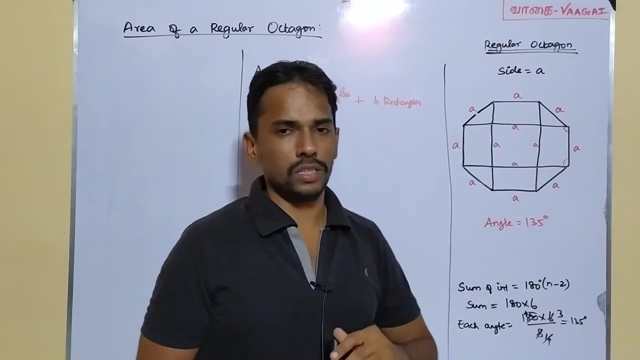 just try to find this sum. and when we are successful in finding this sum, this value, then our task is over. we'll be obtaining the area of the octagon, right? yes, so yeah. the next thing is: let's again have a close look about these triangles and these rectangles. see now if you have a close. 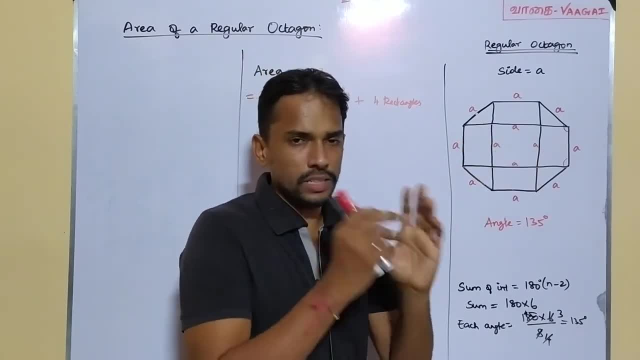 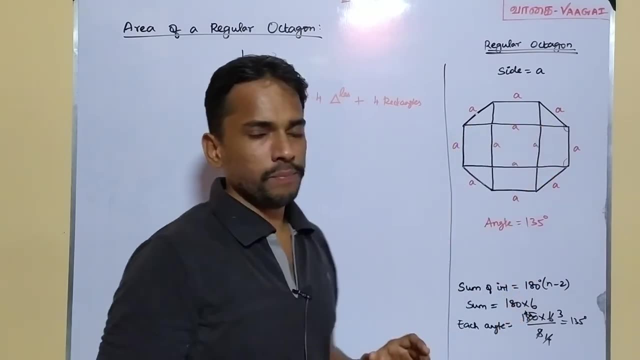 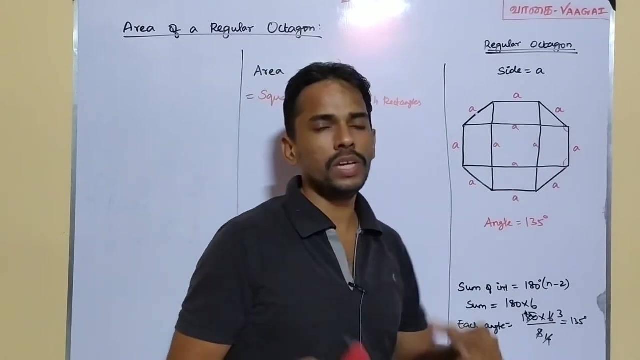 look on these triangles and these rectangles. since we have this octagon to be a regular octagon, what happens is this: triangles will also be congruent. i mean, all those four triangles will be same size and all those four rectangles will also be of the same size. so that means just, we can just take it. 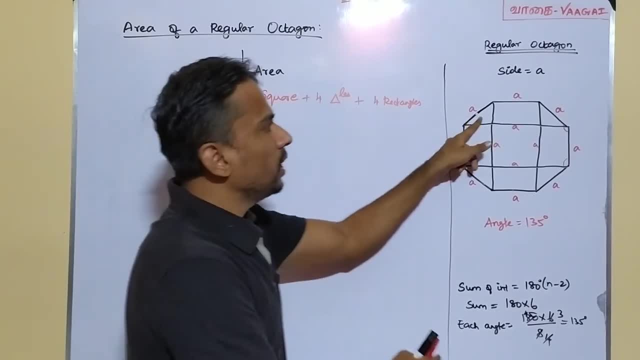 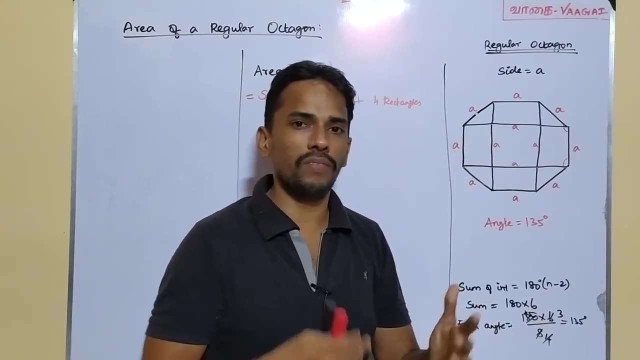 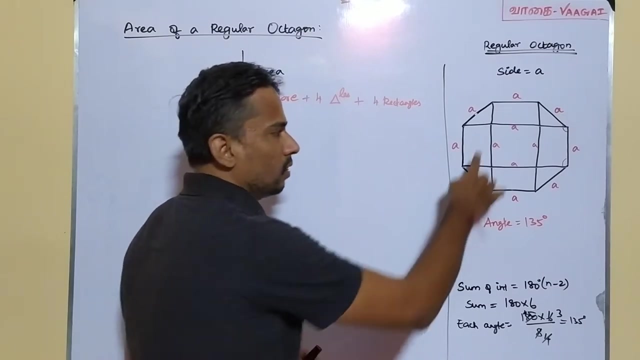 take it like square plus four times of any one of these rectangles area plus four times of any one of these rectangles area. is the point clear? so that way we can do we'll be able to get the answers. so, coming to the squares part, it's very clear: square. we just realized that the side of the 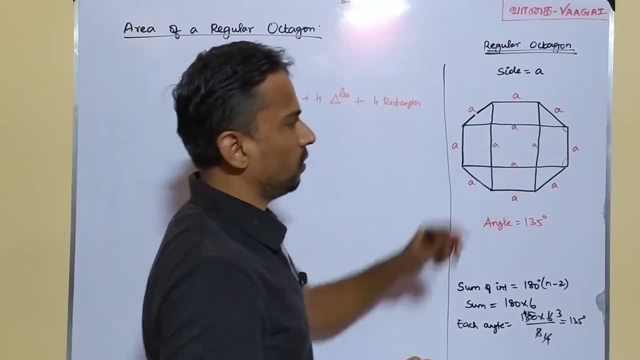 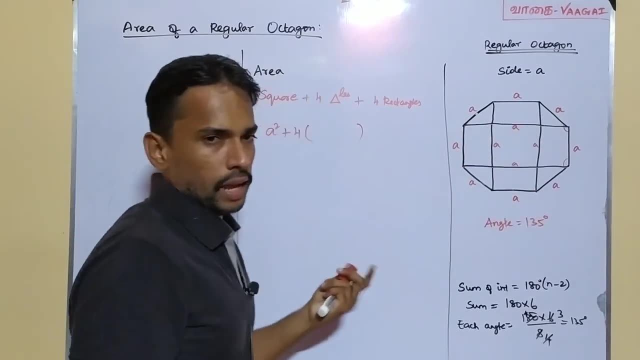 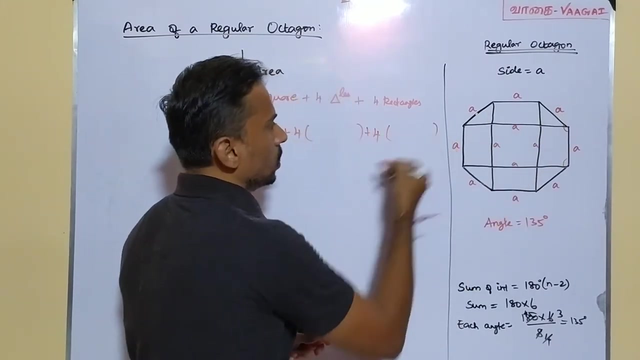 square is a, and in that case, area of that square will be a, and in that case, area of that square will be a equal to a square, plus four times of area of any one of these rectangles, plus four- i mean this triangle- and four times of area of any one of these rectangles. okay, right, so now all we need is: 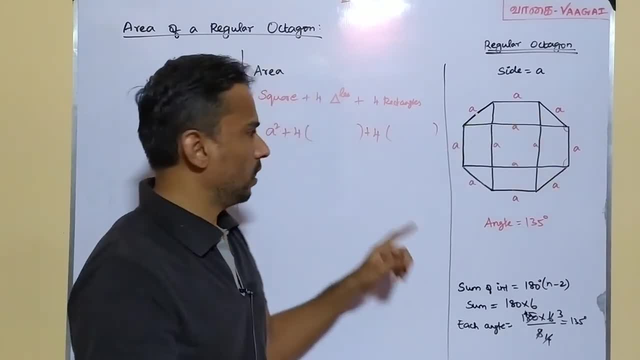 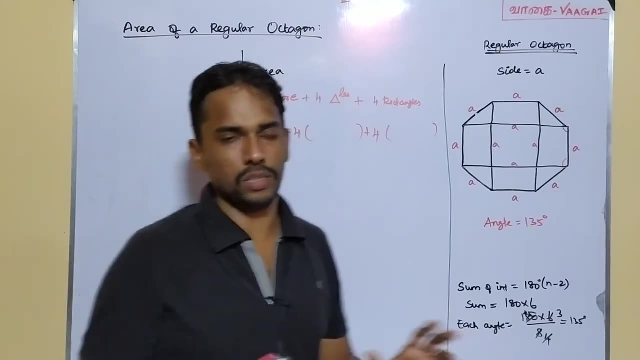 area of any one of these triangles so that we can place it here, and area of any one of these rectangles. if we find that, that we can place it here, and we simplify and get the answer: is it or not? yes, so our next objective is going to be: 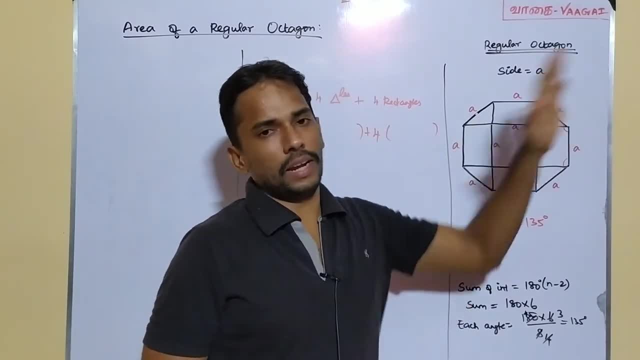 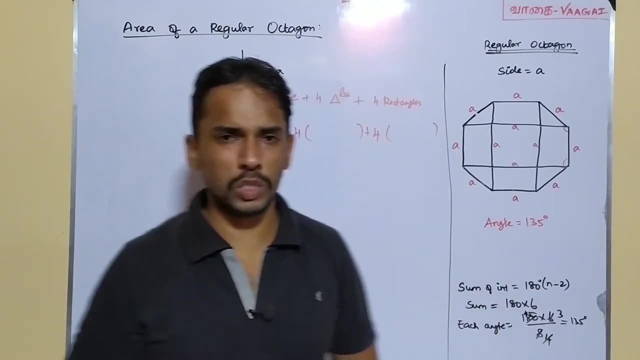 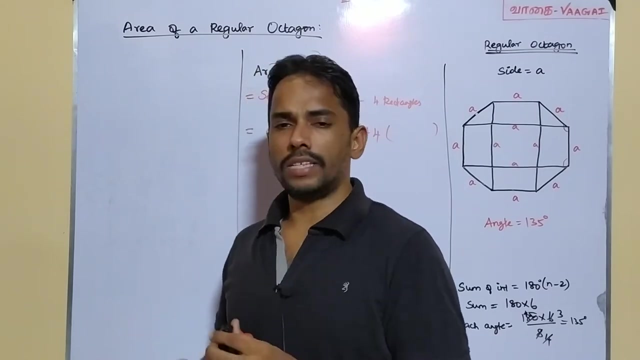 finding this area of these triangles and rectangles. that's what it's going to be right? okay, so we have some empty space here. let's try to use this space now in order to find the area of this triangle and also rectangle. yes, fine, yes, ready. so for that reason, what let me do is i will just 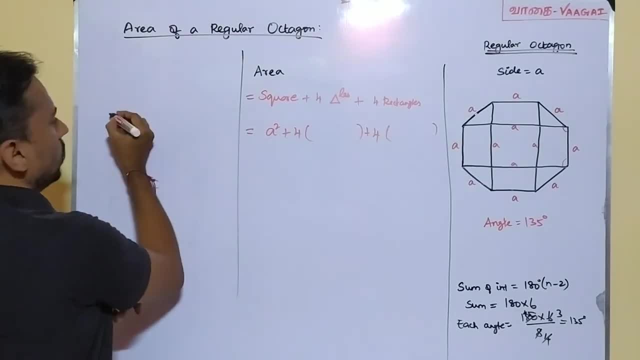 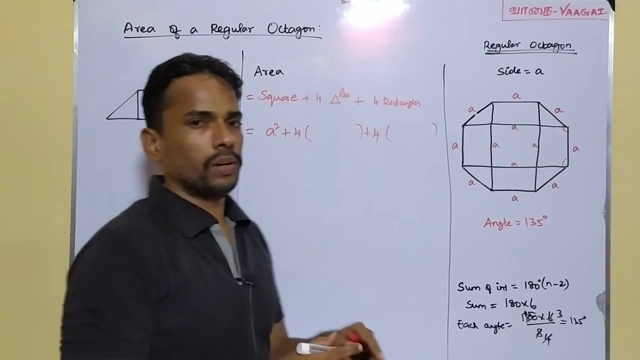 redraw the same shapes here, so i'll just draw a portion alone here. so we have this corner having a rectangle- i mean a triangle- and we have a rectangle which is attached to it. okay, so we know that all four triangles are same shape, they have the same shape and all four rectangles also. 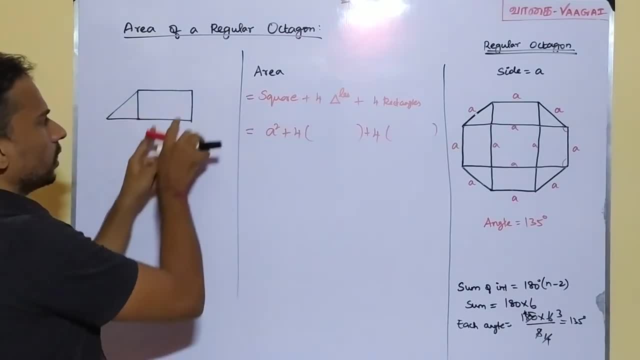 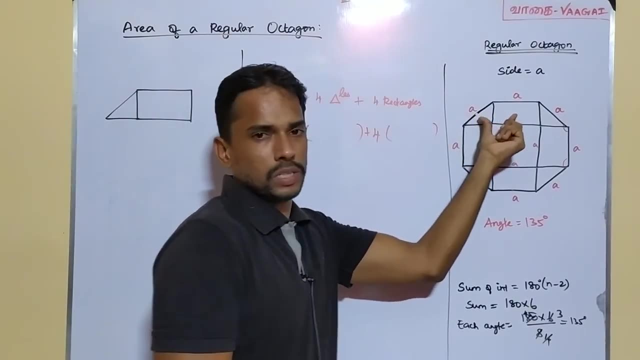 have the same shape. for that reason, i'm just considering only one triangle and only one rectangle which are touching each other. that's it. okay, i mean this piece and this piece, the top two pieces is what. i'm redrawing it here and we'll just try to observe the property, to find their 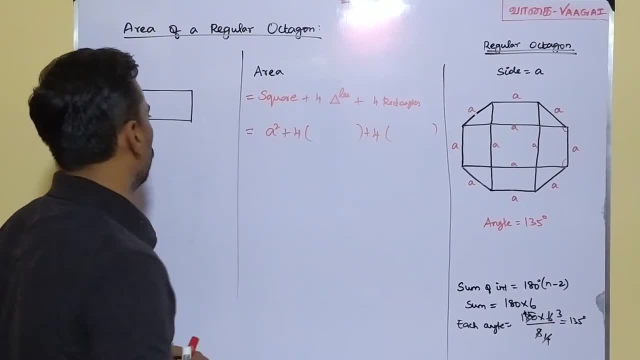 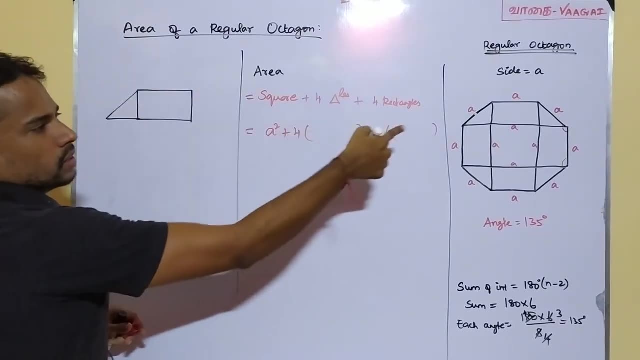 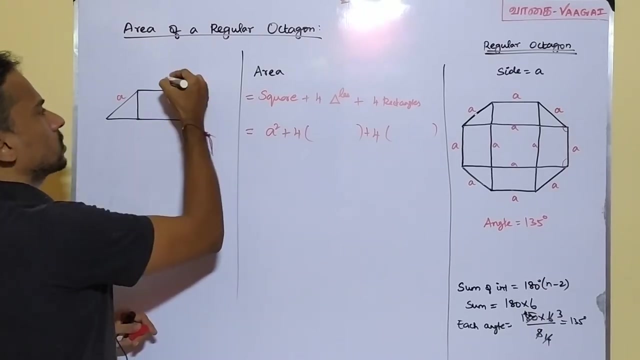 areas so that i can place it here to complete our derivation. okay, yes, so here. what we know is this: this portion of our triangle is having its side to be a, and this top portion of our rectangle, i mean one length of the rectangle, is again a fine. yes, and we also know that area of the triangle is equal to half. 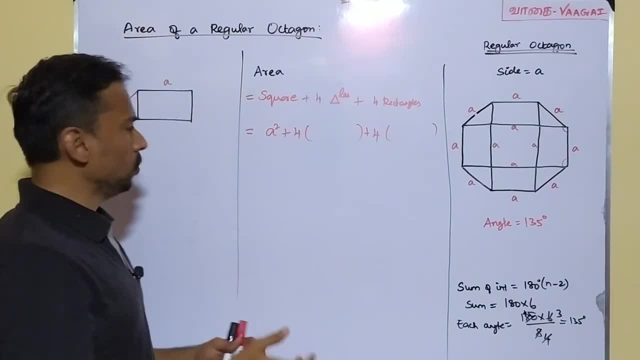 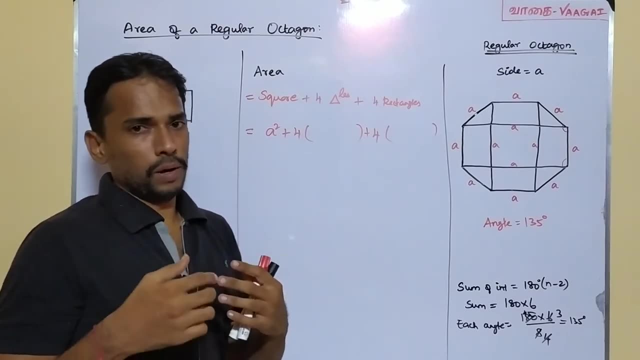 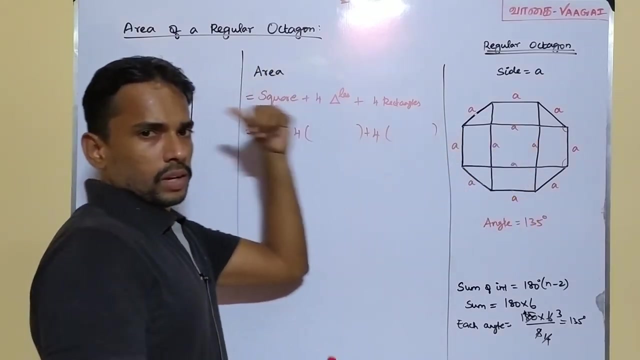 into base, into height, and area of the rectangle is equal to length into breadth. is it so if we, If we know that we will be able to get the answer, but unfortunately our values are incomplete, Let's again try to see, have a close look, then complete those things so that we can. 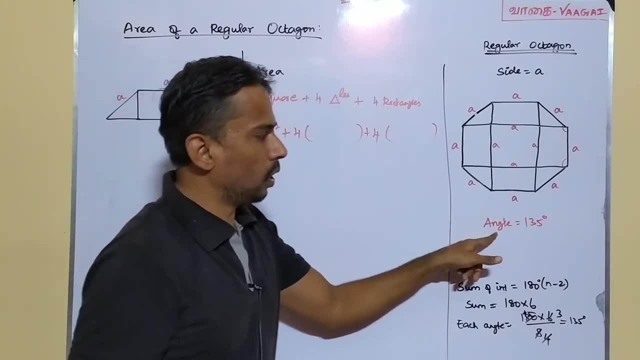 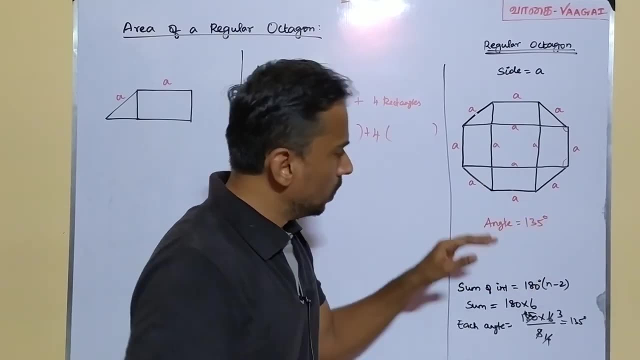 get those areas fine. yes, and come back to our angles part. here we have already found that each of these interior angles is equal to 135, is it or not? Let's try to use this information over here so that we will just check whether it is helpful. 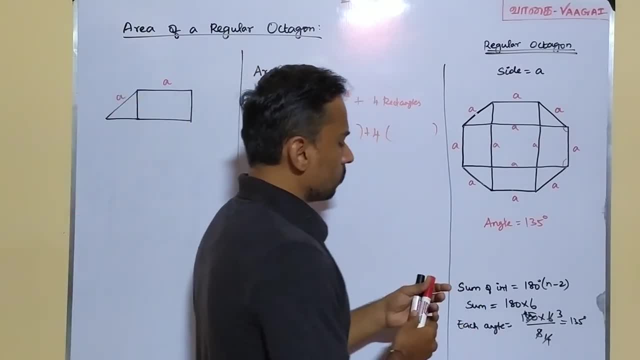 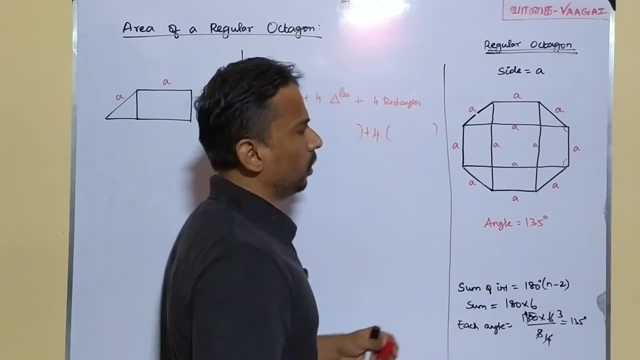 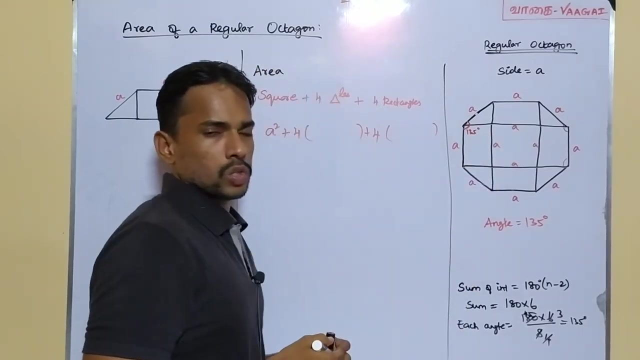 for us to complete what we are hanging with. So, yes, and what we can do here is: yeah, just take this one of these angles to be 135, so if I consider this angle to be equal to 135,, fine, alright. So what happens is we clearly have this 135, this angle 135 that is seen here inside that. 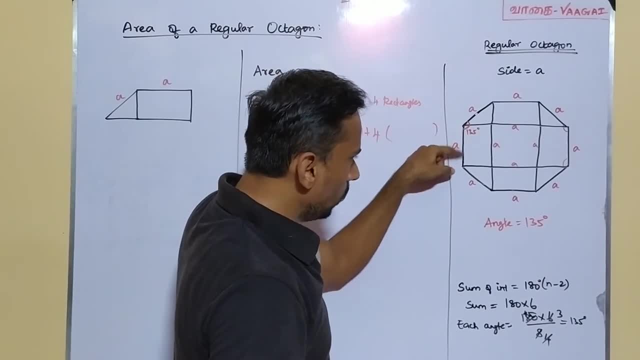 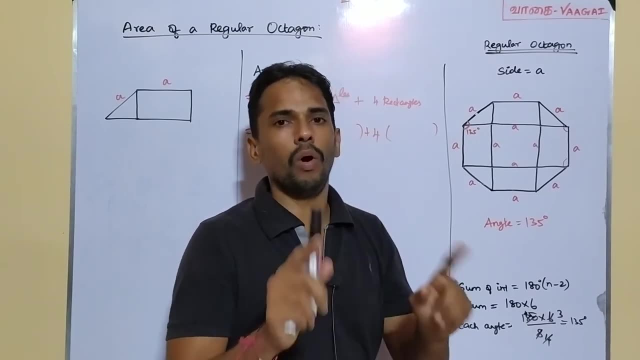 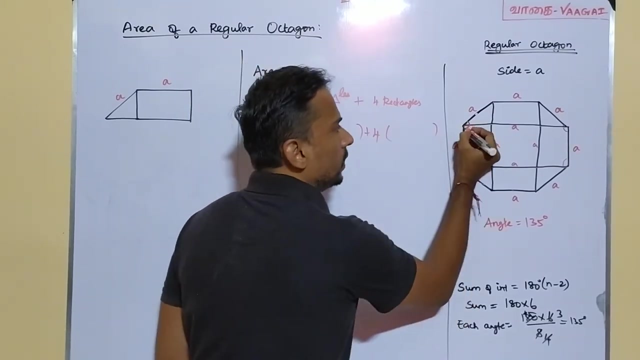 interior angle is being shared by exactly one rectangle and one triangle, is it or not? And we surely know that inside a rectangle, the corner angle will be always equal to 90 degrees. It is always right angle, right. So in that case, this corner angle will be definitely a Right Angle. it will be a Right. 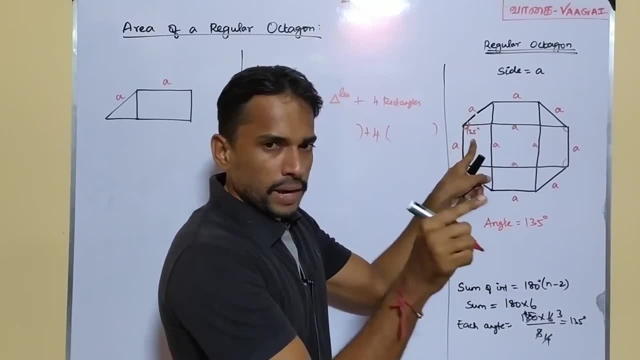 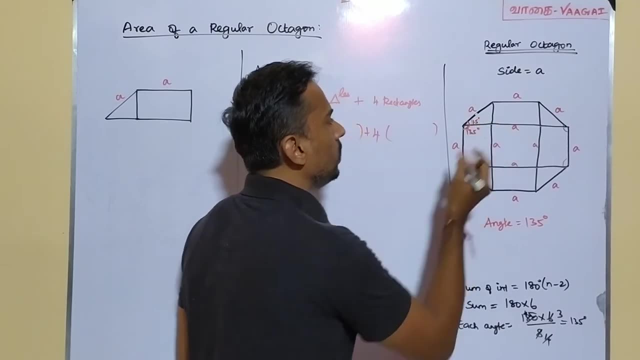 angle. So what we do is just do 135 minus that 90. So that we will have the remaining portion, which will be 135 minus 90, which is 45 that will lie here inside the triangle. so that means we are now very sure with this angle. 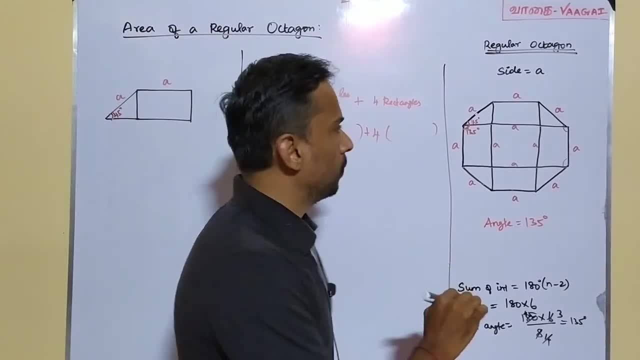 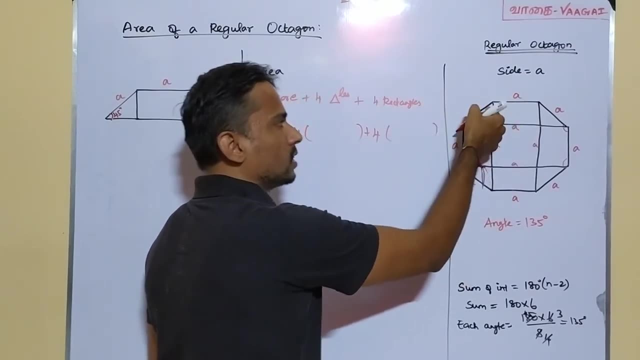 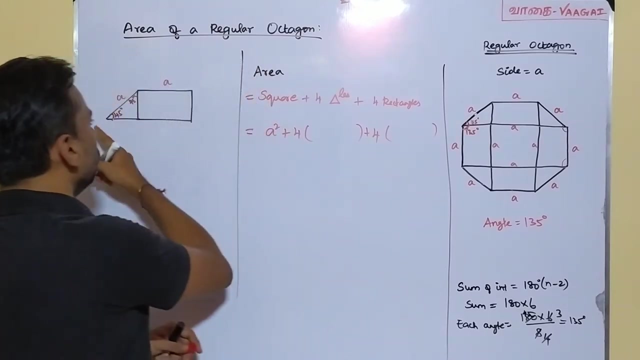 to be equal to 45 degrees. Now I can repeat the same experiment over here. So this full angle will be again 135, where this will be shared with 90, and obviously the other part here, what we see here, will be another 45 degree. I hope the point is clear to you. So we have a right triangle here, actually, and another. 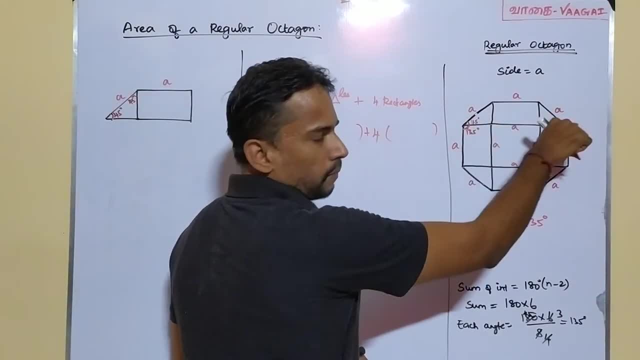 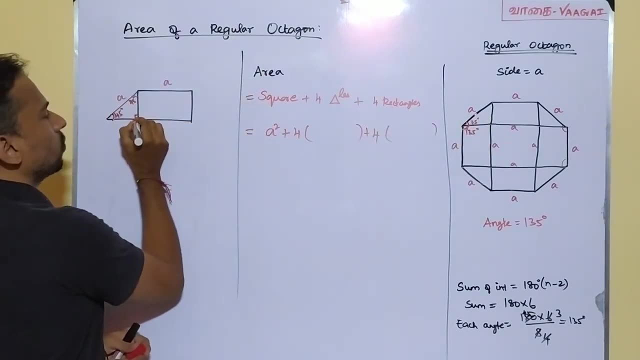 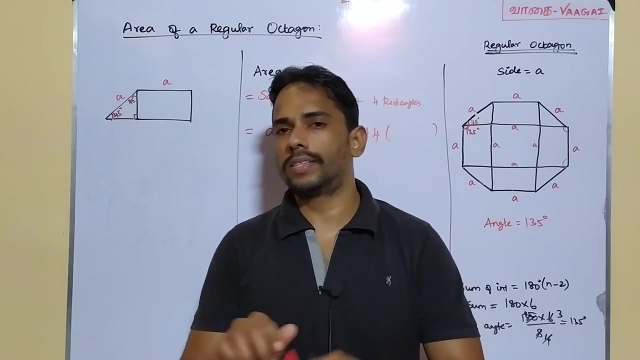 thing is, since we have these sides to be intersecting here with the squares, with rectangle, and we can very easily assure that this corner angle will be again equal to 90 degrees, So that means the triangle. what we see here is a right angle triangle and at the same time it is going. 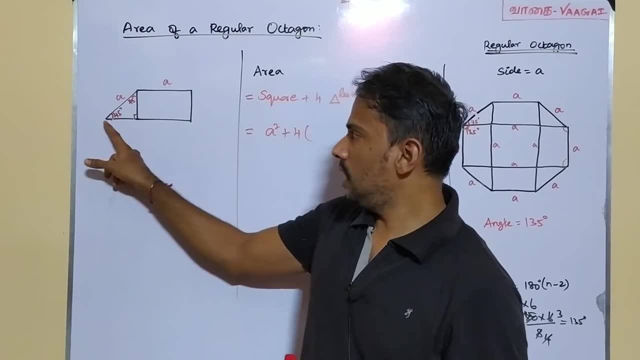 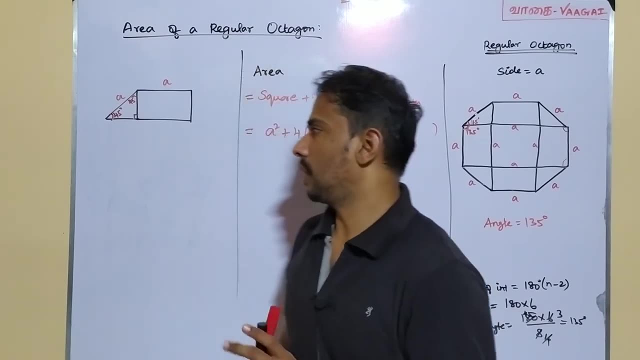 to be an isosceles triangle, because see, here we have two of those angles to be equal. In that case, it is going to be an isosceles triangle, Is it or not? Yes, fine. Now the next part is in an 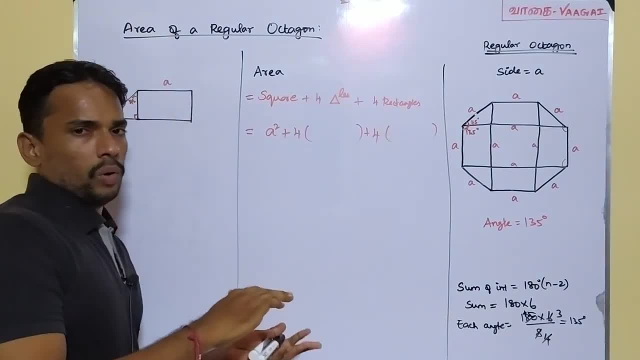 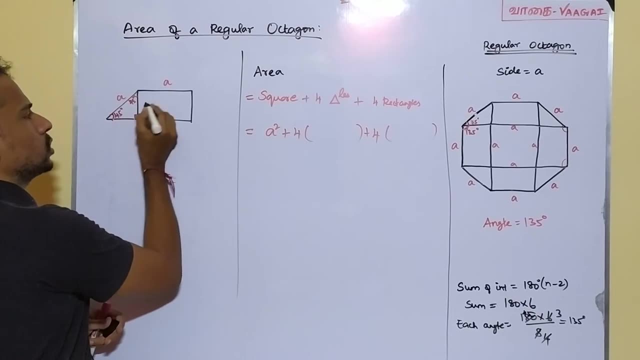 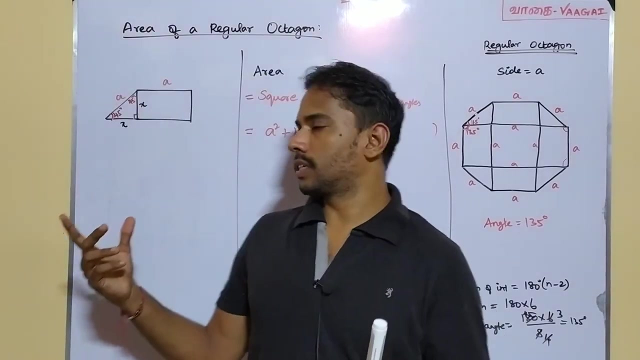 isosceles triangle, there are two angles to be equal. So it implies the two sides will also be equal, Is it or not? So let us have the two sides, these two sides, to be the equal sides, length to be some x and x. Fine, Is it or not? So now our task is: 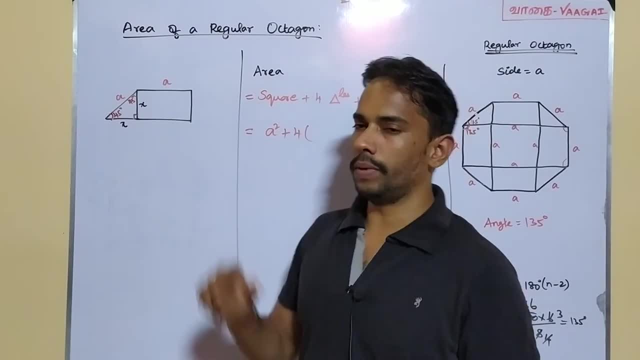 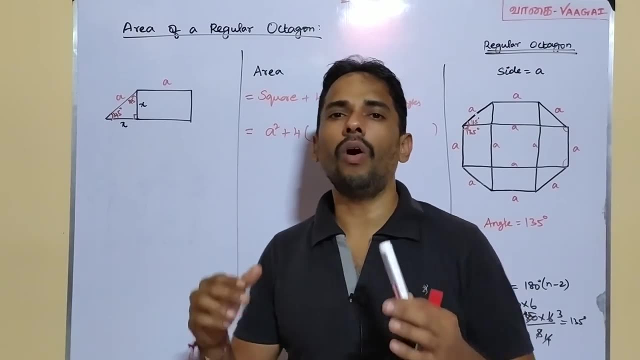 almost over. See, here we have this value to be x and this is to be x. and now what happens is x, x and a. that completes right angle triangle, and we all very well know Pythagoras theorem. So, with the use of Pythagoras theorem, 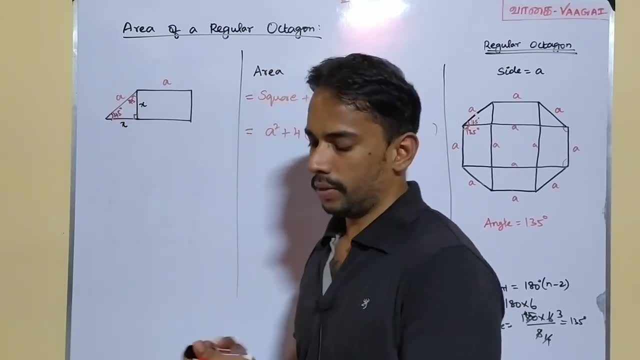 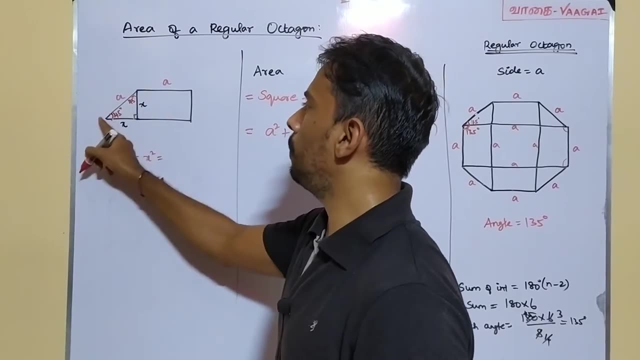 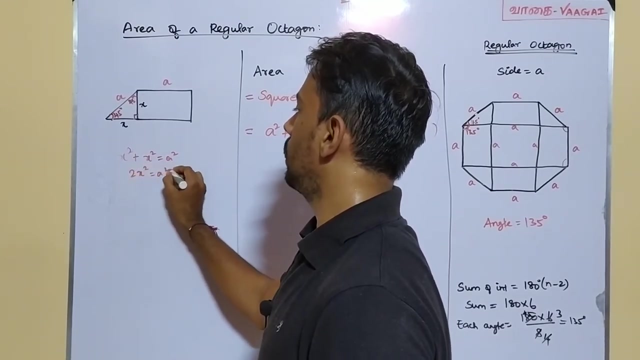 Let us use or let us connect these three sides, so that what happens is we will be ending up with this x square plus this x square will be equal to our hypotenuse of a triangle, which is nothing but a, So a square, so that we get 2 x square is equal to a square and which gives x square is. 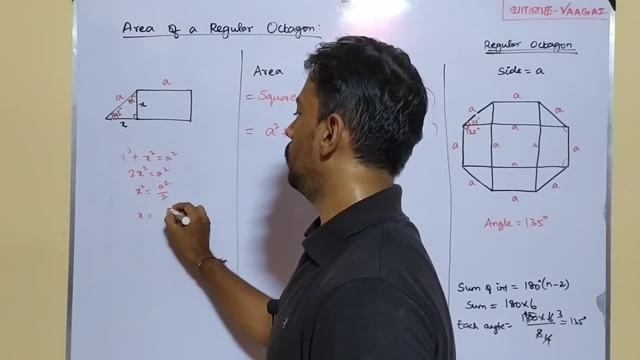 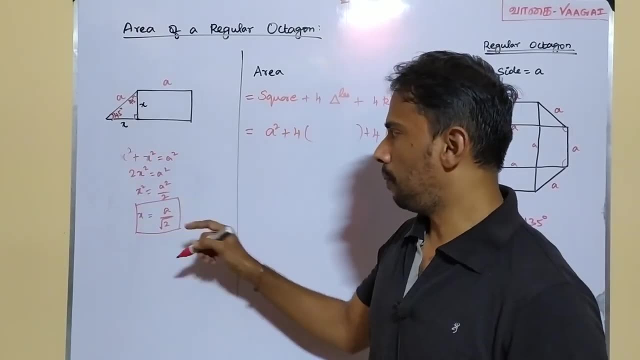 equal to a square by 2, and that gives x is equal to a by root 2 when we take square roots on both sides. So we successfully got the value of x to be equal to a by root 2.. So let us connect these. 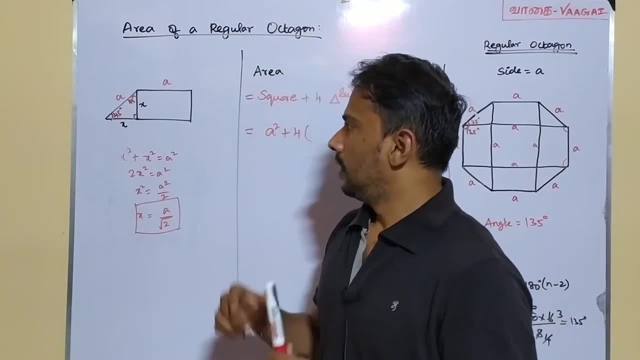 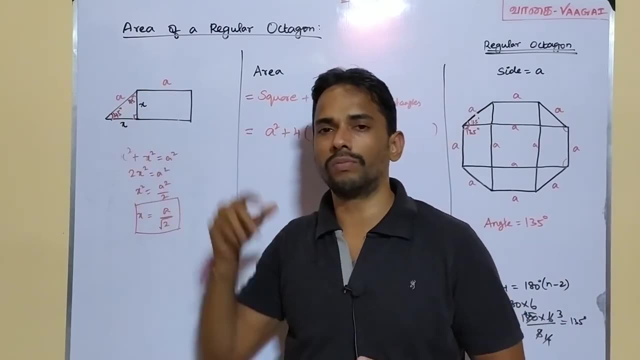 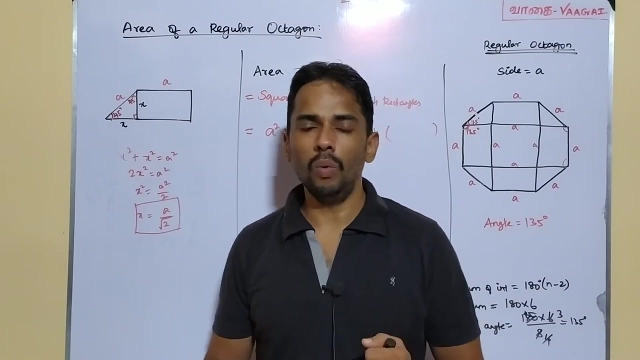 two sides. So that is it. and the other happy news is that this breadth of this rectangle is again same as this height of this triangle, Is it or not? So, in that case, this breadth of this rectangle is once again the same x value only, and now we are very successful that we are having all the values. 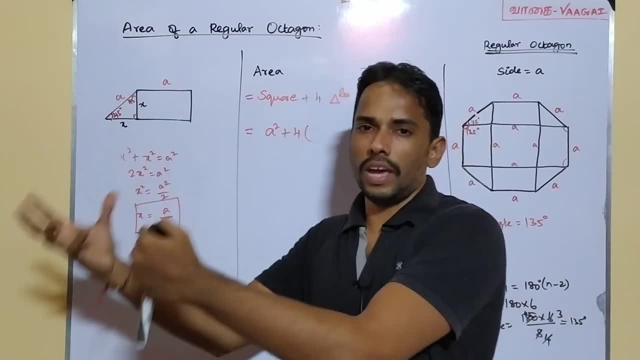 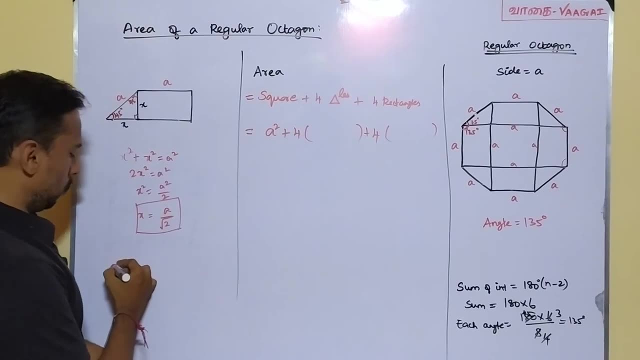 all the required values that we, that that are required to find the area of both the triangle as well as rectangle. Yes, right, So yes, let us complete the process Now. the area of the triangle will be is equal to: we know the area of a triangle's formula: half into base, into height, So half into, so our base and height are. 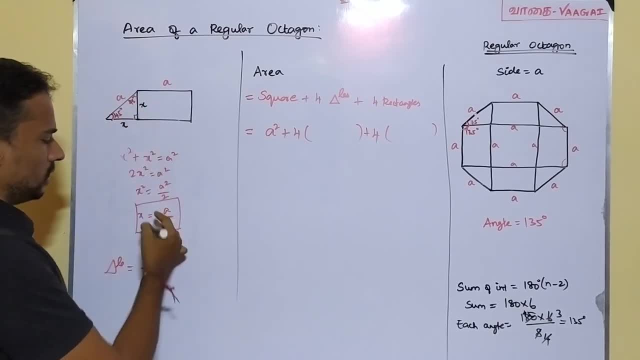 nothing but x and x only. So in that case it will be a by root 2 times a by root 2.. So this completes our value to be equal to 1 times a times a, which is a square by come to the denominator we have. 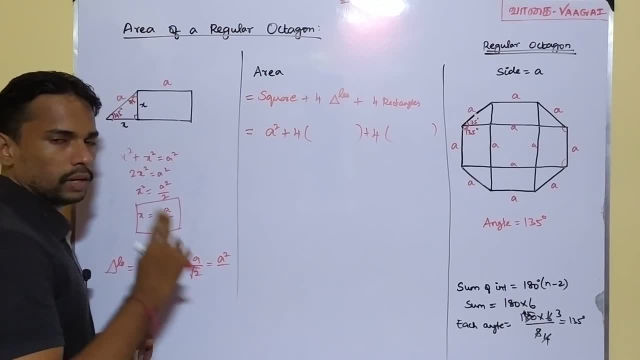 2 into root, 2 into root 2.. So root 2 is equal to a by root 2.. So this is equal to a by root 2.. So root 2 into root 2 will give us 1, 2 and 2, 2's are will be a 4.. So that means area of one triangle. 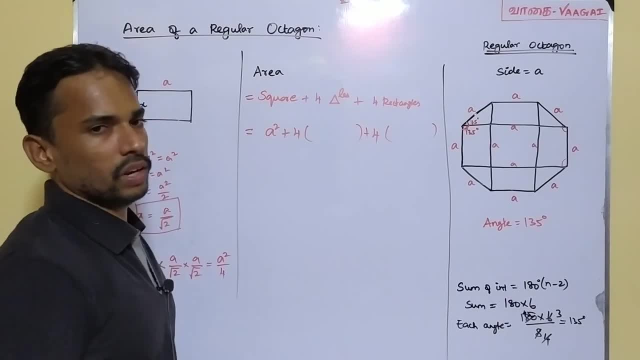 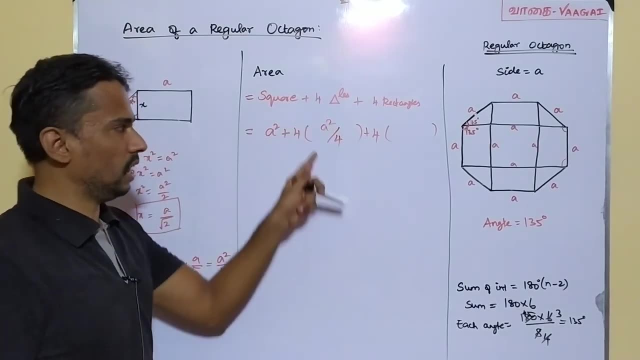 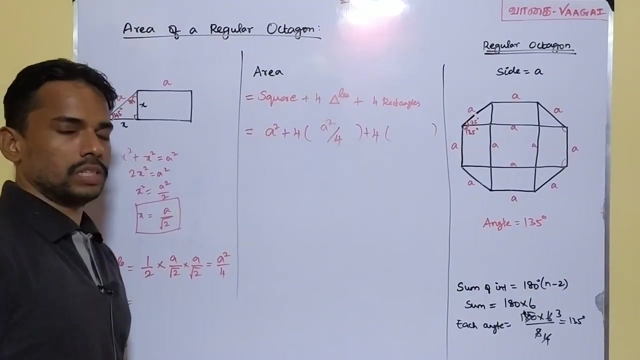 one of these triangle will be equal to a square by 4.. So we can very well substitute this value over here so that we get a square by 4 here, because 4 times of triangle's area is what we have, So 4 times of a square by 4. and next is come to the rectangle here. So rectangle's area is none other. 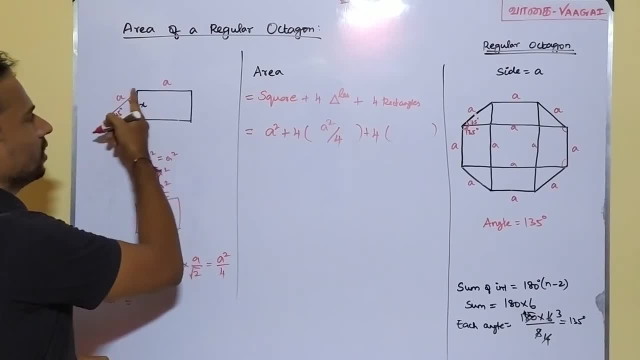 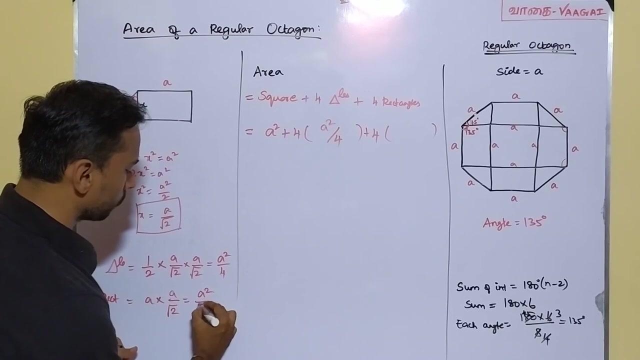 than length into breadth, Is it or not? So our rectangle's length is already available Here. it's nothing but a times our breadth is this x, which we just found out. So a by root 2.. So that we will get rectangle's area to be equal to a square by root 2.. And now we can very well substitute. 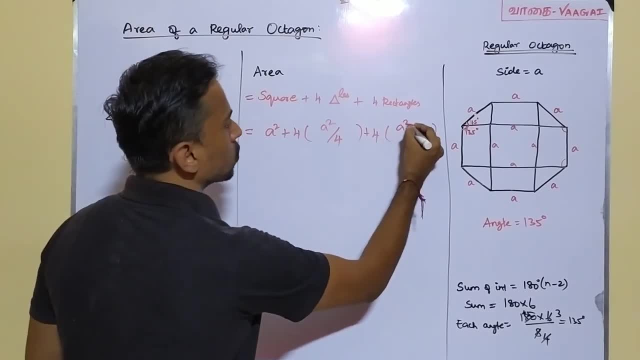 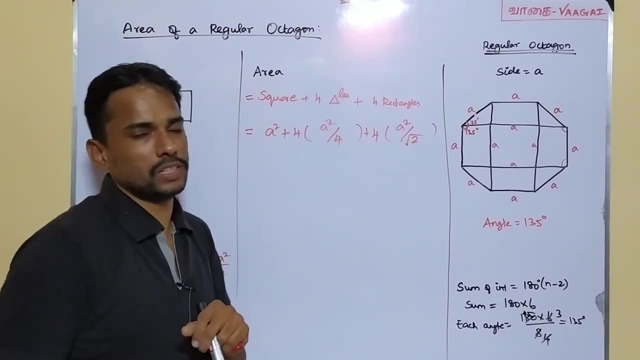 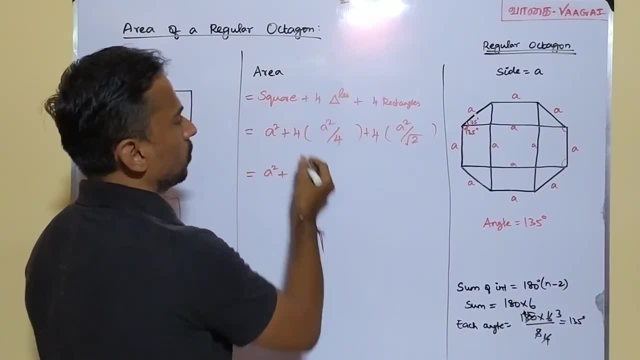 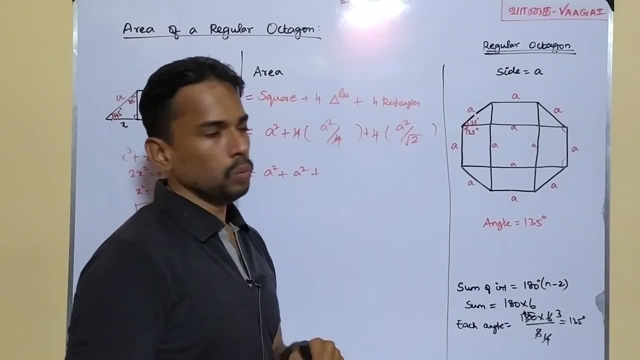 plus 4 times of a square by 4, which will be nothing but 4 and 4.. They gets out So we will end up with a square plus. Here we have 4 times of a square by root 2.. So this 4 by root 2 can. 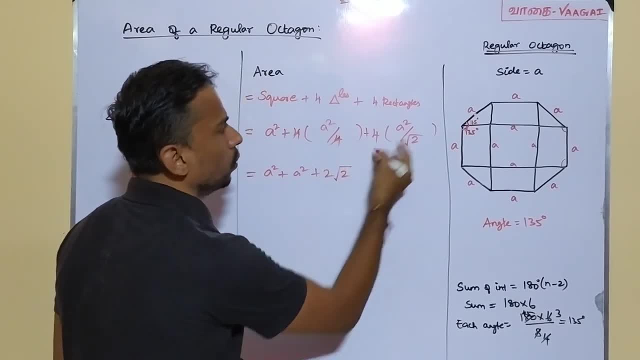 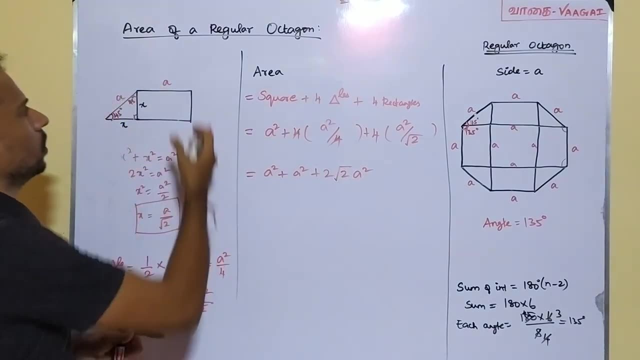 be written as 2 root 2.. Is it or not? So this is 2 root 2 a square. You may ask how it works. So if you want, I can just show that explanation over here. So somewhere over the top here, because I. 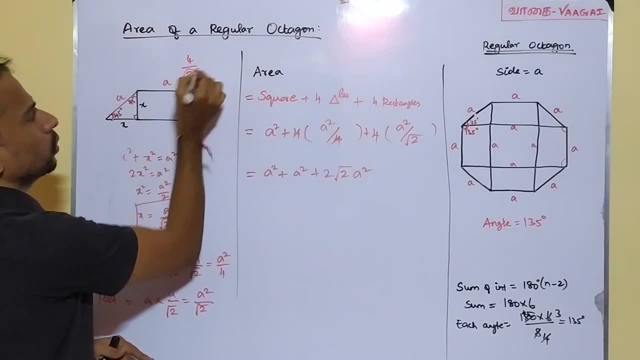 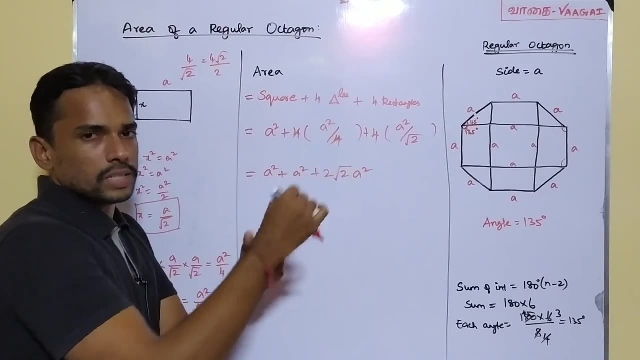 have some empty region here, So 4 by root 2.. Actually 4 by root 2 can be written as 4 root 2 by 2.. Is it or not? Why? Because I multiply root 2 and root 2 in both numerators. 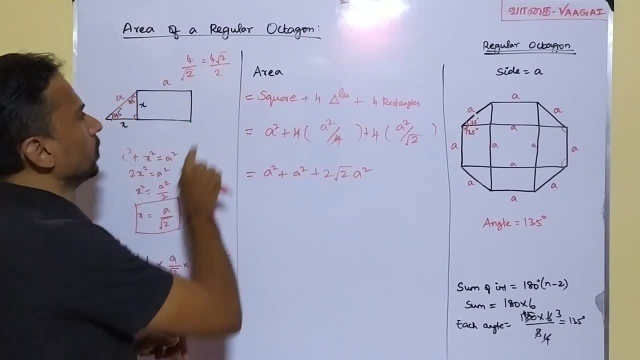 and denominators. So 4 root 2, it becomes a numerator, And root 2 times root 2 will become 2.. And now it is very easy for you to realize that this value is none other than 2 root 2.. 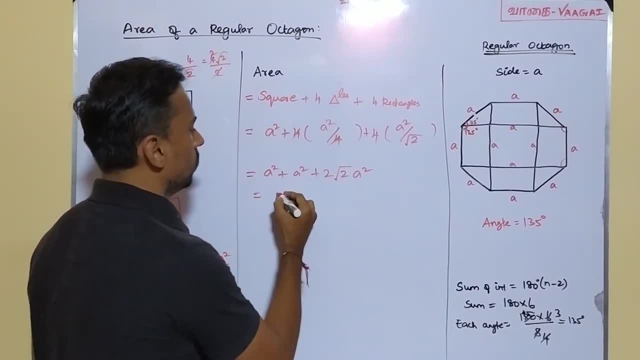 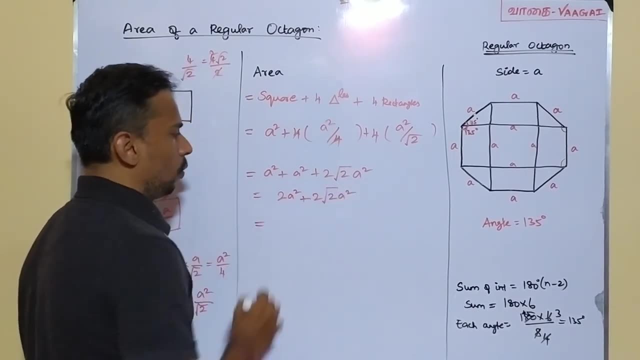 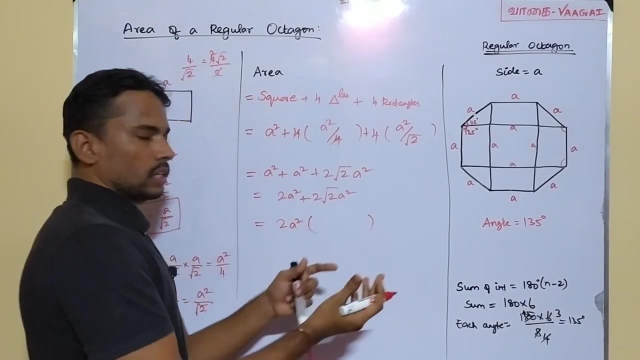 Right, Yes, Fine, So that means we have 2 a square plus 2 root, 2 a square. Fine, Yes, That is it. And now all we need is we can just take the common factors outside, so that we will be having 2 a square as a common factor outside. We can just remove it out, so that all 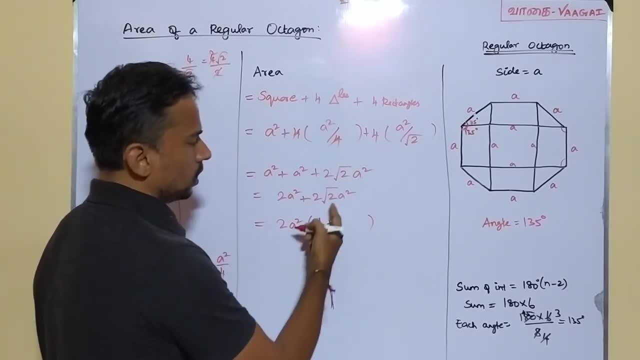 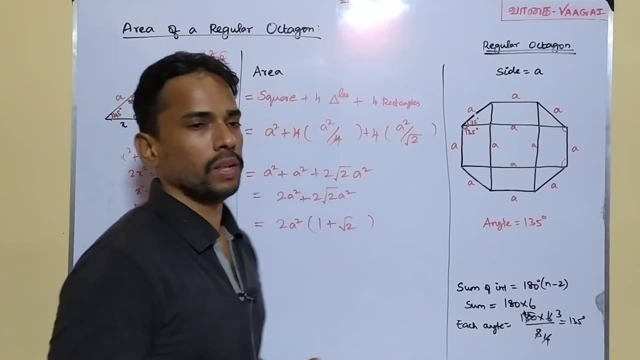 we will be having inside is 1 here plus a root 2 here. So that means area of a regular octagon whose side is a is given by the formula 2 a square times of 1 plus root 2 or 2 a square of. 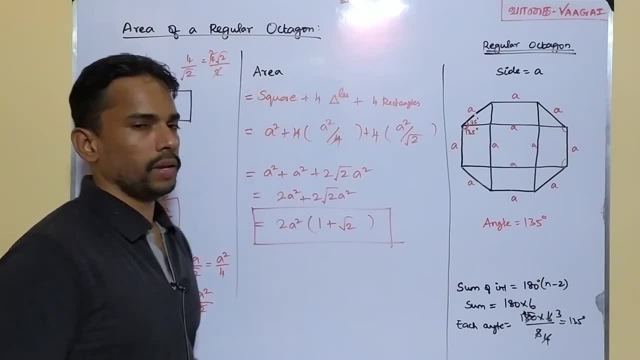 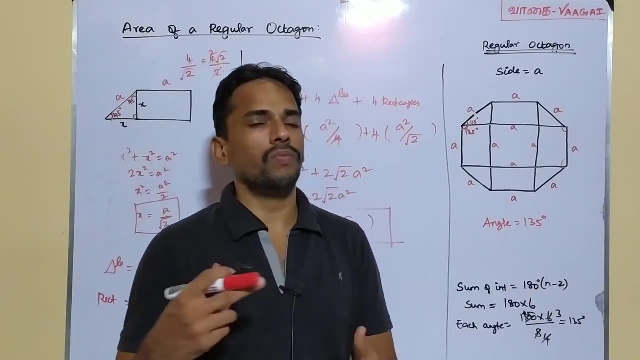 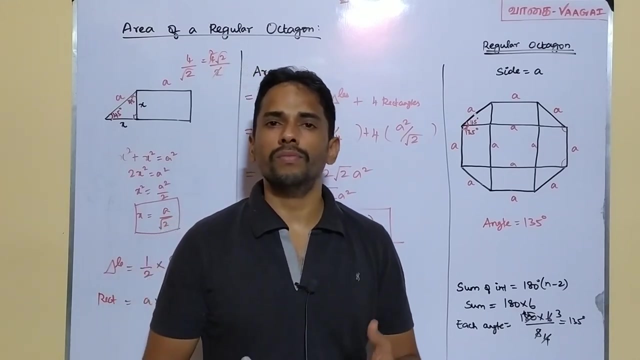 root 2 plus 1, because addition is commutative. So this is going to be our formula to find the octagon. I hope this derivation, what we have done, is very clear to you And if any doubts you are most welcome to comment it here in the comment box. And again very soon in the 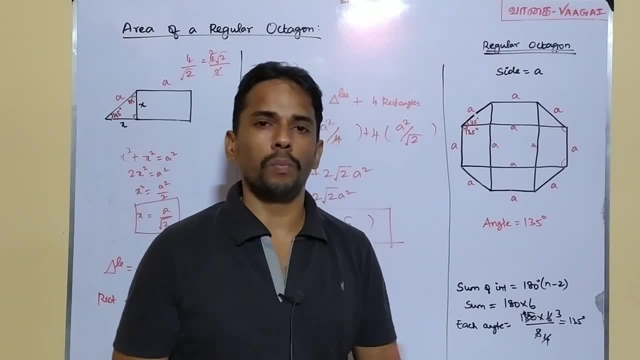 next session. let us catch up with some other interesting concept or problem very soon there. Thank you so much, Bye.